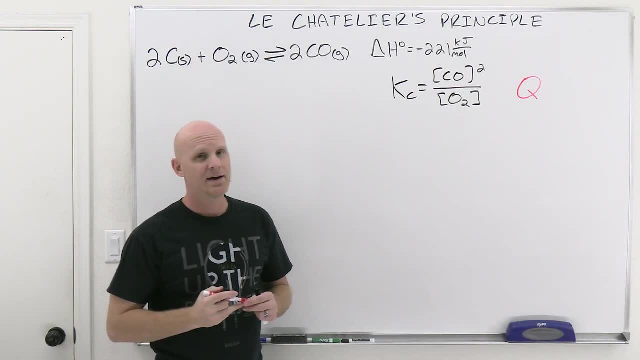 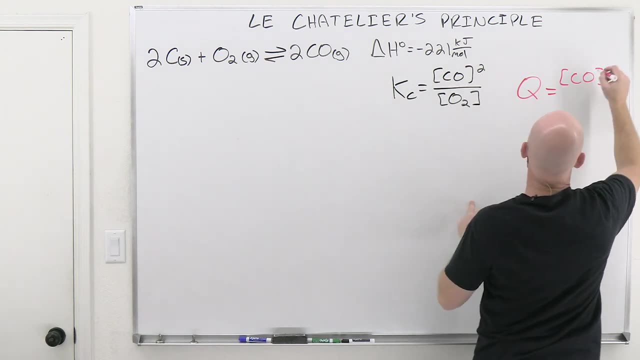 quotient we alluded to in the last lesson. it's represented by the letter Q and it's equal to the ratio of products to reactants here in a reaction. So for the one we've been dealing with and we're dealing with again here, it's equal to the ratio of products to reactants. 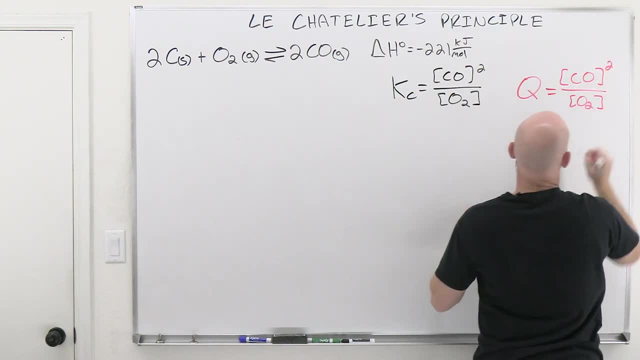 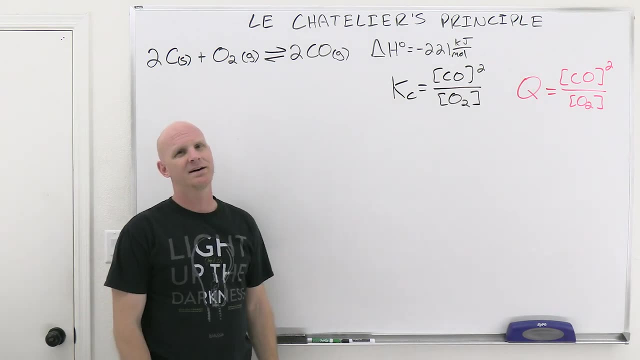 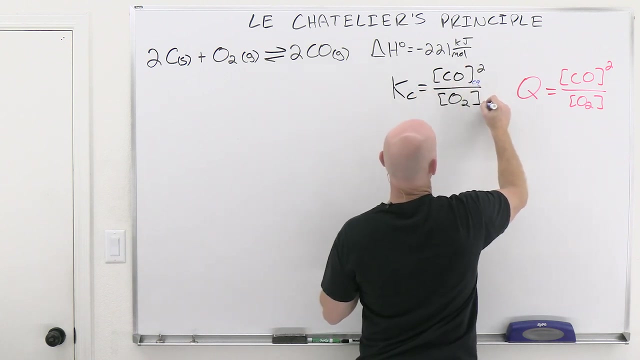 So we have an issue You might be like. well, Chad, that's the same ratio as K, It is. The big difference is this, though: is that for this ratio to equal K, you have to have to have to be. 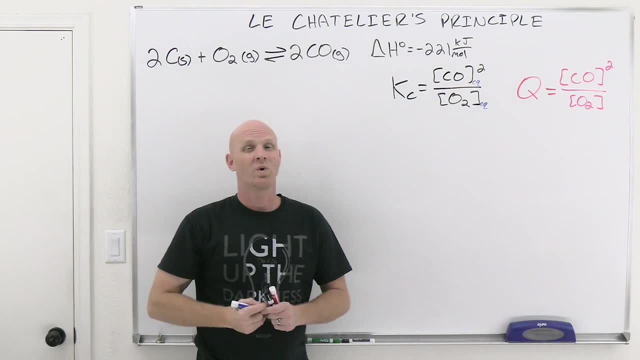 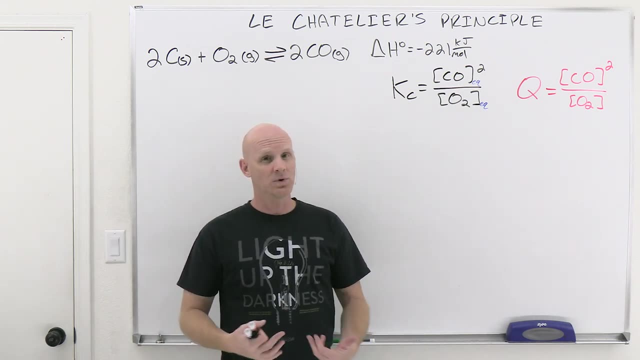 measuring these concentrations at equilibrium, Whereas in general, this ratio is always equal to Q, whether you're at equilibrium or not. And so if you're at equilibrium, then this ratio is equal to both Q and K, because that's the point where Q and K are equal. However, if you are not, 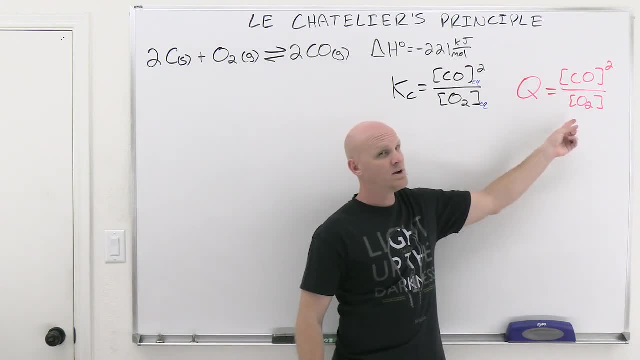 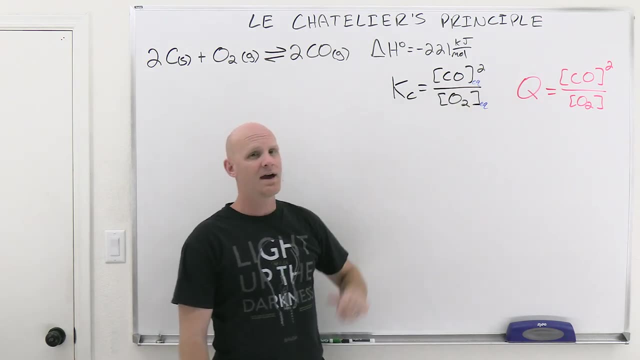 at equilibrium. if a reaction is not reached equilibrium, then this ratio equals Q, but it does not equal K. This will be important. It turns out comparing the value of Q and K is a great way to look at Le Chatelier's principle, but just one of the ways, All right. So if we take a look at 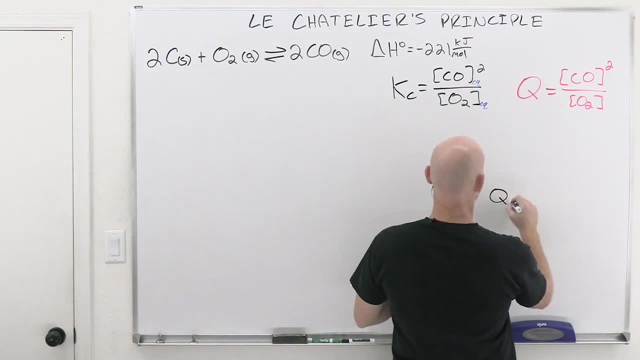 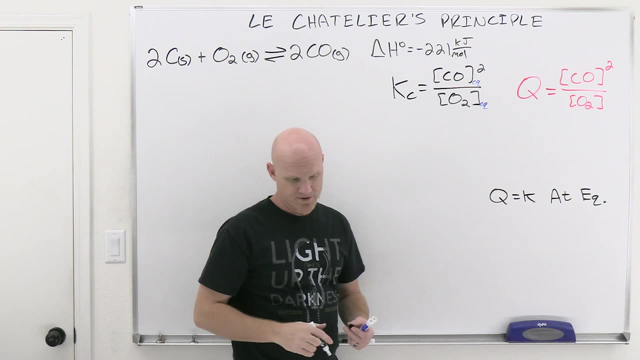 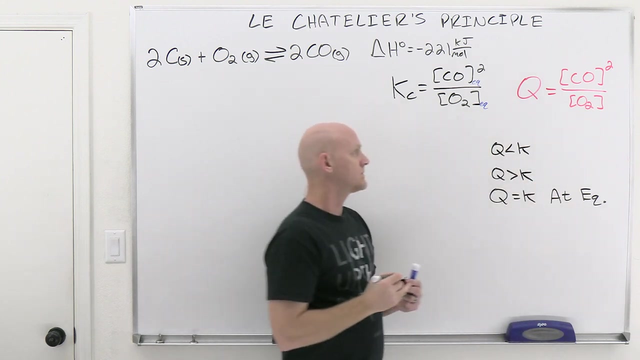 what's going on here? we can talk about Q equaling K- and that is true for reaction that is actually at equilibrium. But what if you're not at equilibrium? So what if Q is equal, less than K or greater than K? So then what's the deal? So well again, if Q is either bigger or smaller, 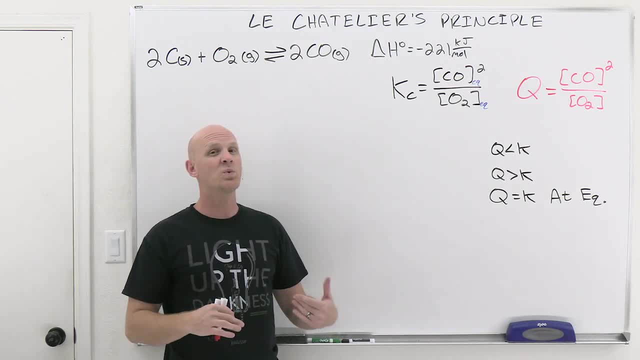 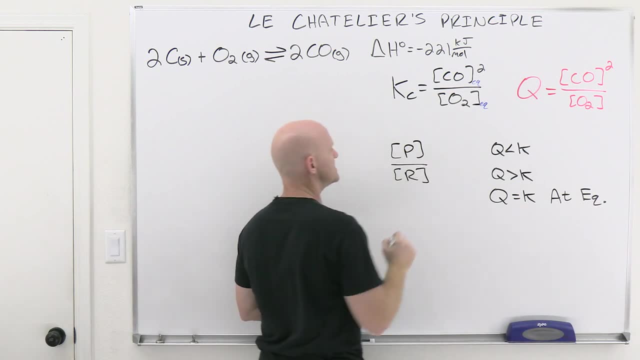 than K, you're not at equilibrium. but you know more than that. You can actually figure out which way it needs to shift to get to equilibrium. So again, we're looking at this ratio of products to reactants and I'm just going to look at it very generically here. Leave off, you know any. 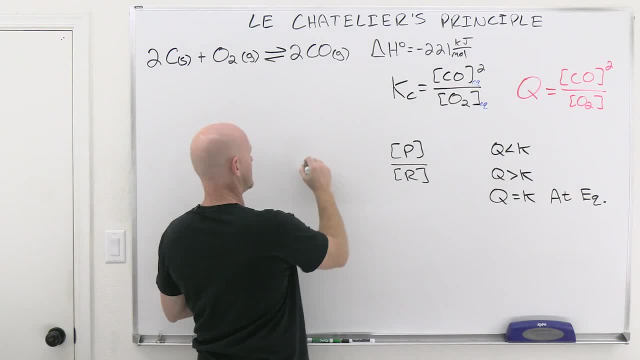 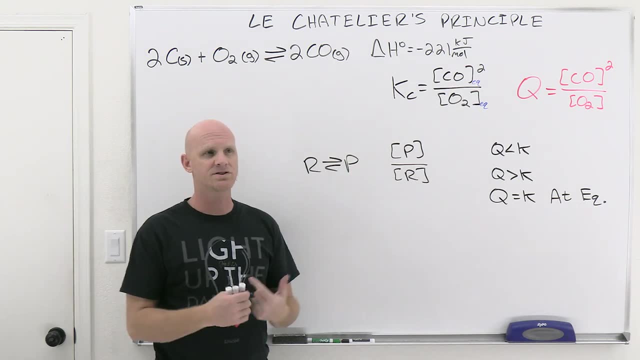 kind of exponents or anything like this. but we have reactant, we have product and we have a reaction where we've got reactants converted to products. So- and this ratio here can change As the reaction proceeds- this ratio is going to get closer and closer and closer to equaling K. 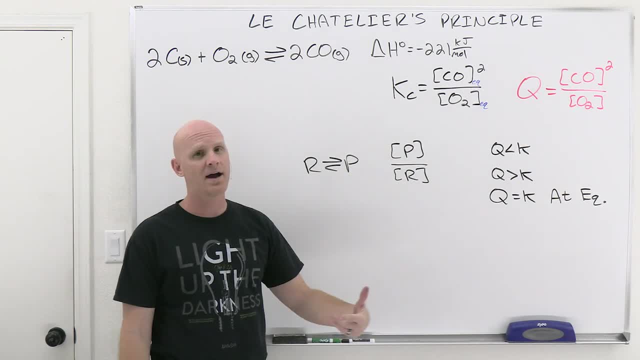 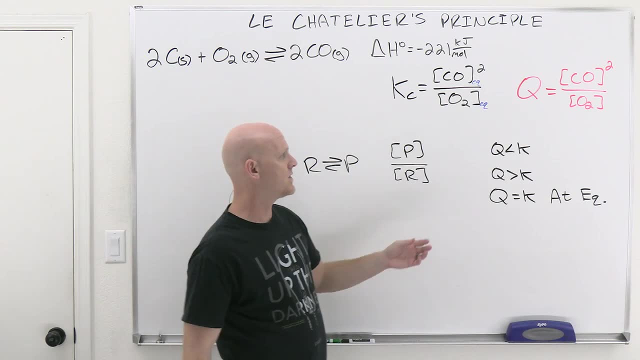 until you finally reach equilibrium, at which point this ratio would exactly equal K. But you find over time it's going to get gradually closer and closer and closer to equaling K, And so you go from a situation where either Q is less than K or Q is greater than K. 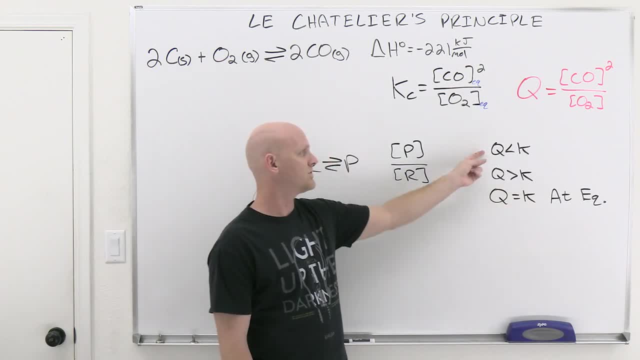 and eventually, either case, you're going to end up with Q equaling K. So notice, let's start with Q is less than K, So let's start with. Q is greater than K, So let's start with Q is greater than K. 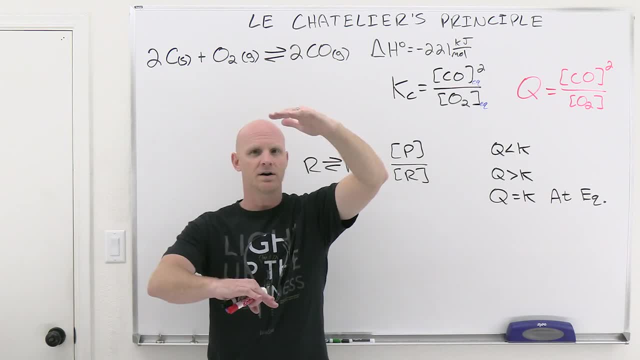 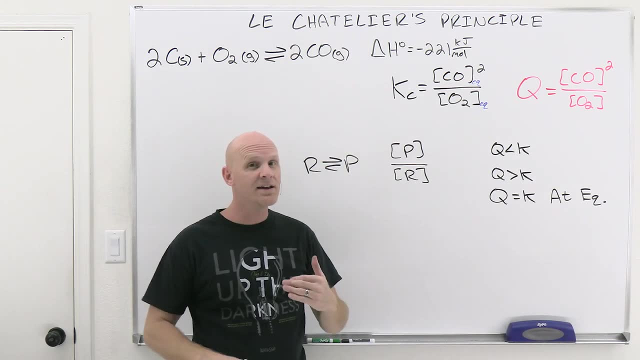 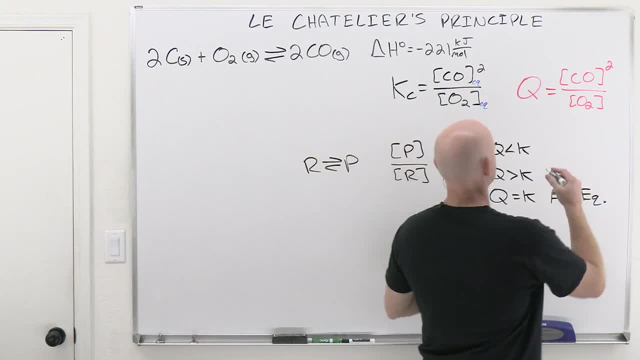 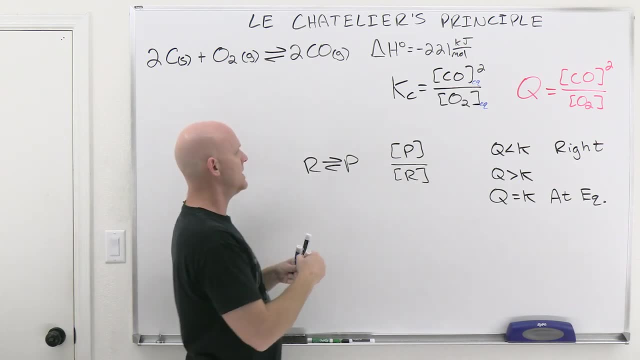 and it's got to get bigger And for Q to get bigger, so that reaction has to shift to the right, we say. So you can kind of take a look at this. So what we mean by shift to the right is meaning that reactions are going to be converted into the products from left to right. 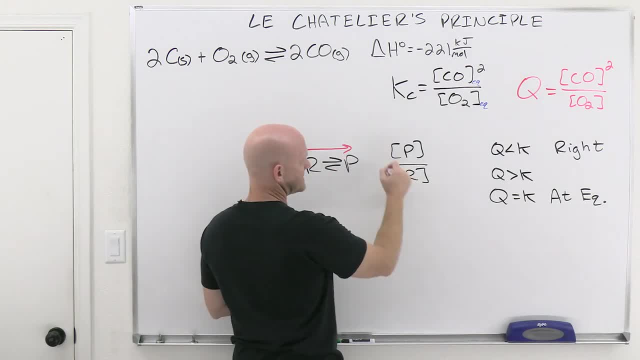 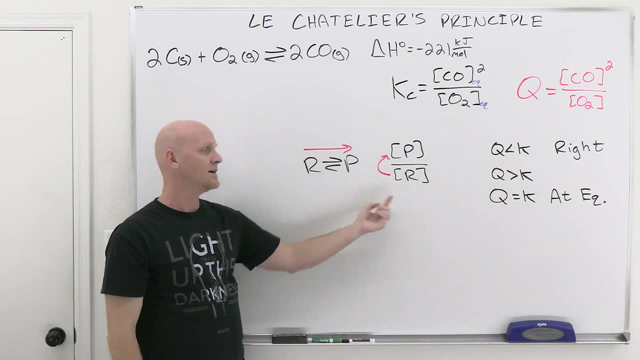 as we normally read, a chemical reaction. And so, if you notice, what that means in this ratio is that you're converting reactants into products. Well, as you convert reactants into products, you're using up the reactants and their concentration is going to go down. So 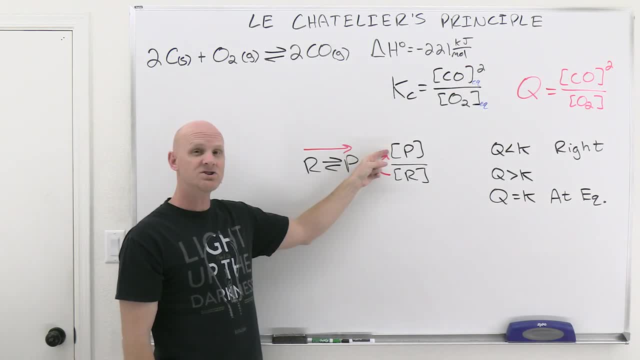 your denominator is going to get smaller And you're converting them into products, so the product concentration is going to go up, so your numerator is getting bigger. Well, if your numerator is getting bigger and your denominator is getting smaller, then overall this ratio is going up. And it's going up again because right now, 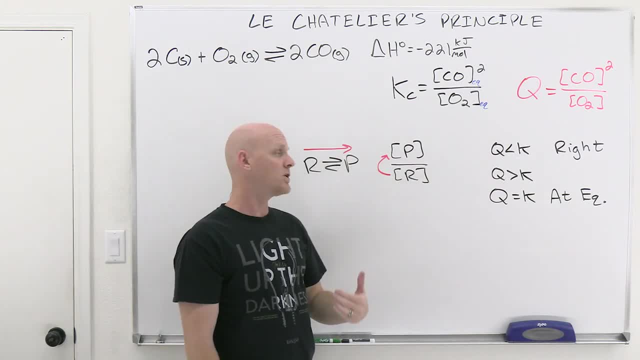 it's too small, It's less than K and it wants to be equal to K, And the only way that's going to happen is if that ratio gets bigger, And that happens if this equilibrium is going to shift to the right. we say: Now, what if we've got the exact opposite scenario, So where we've got Q, 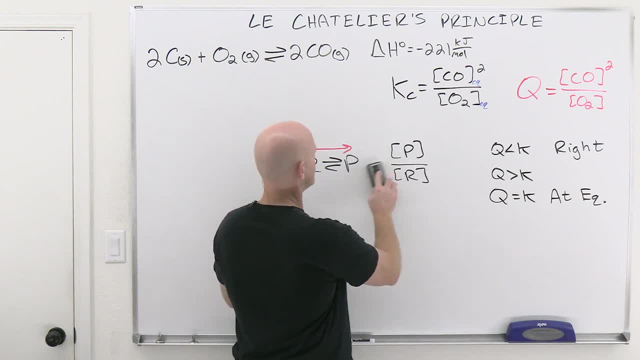 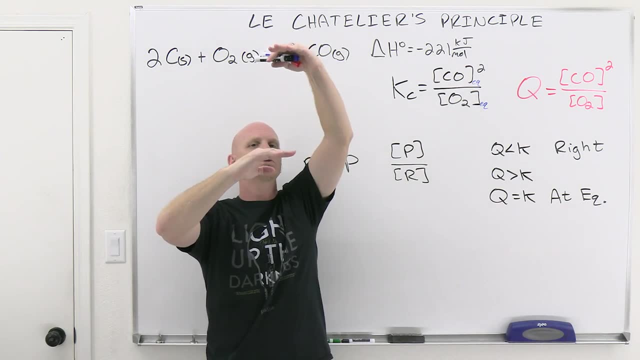 greater than K. Well, if we've got Q greater than K, now Q is too big. So K again is here, but now Q is way up here And over time we're going to find out that this Q value is going to. 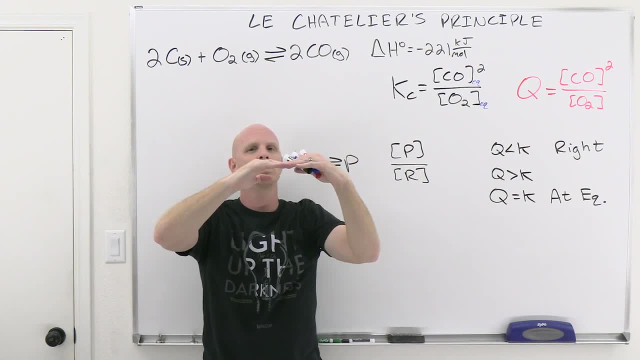 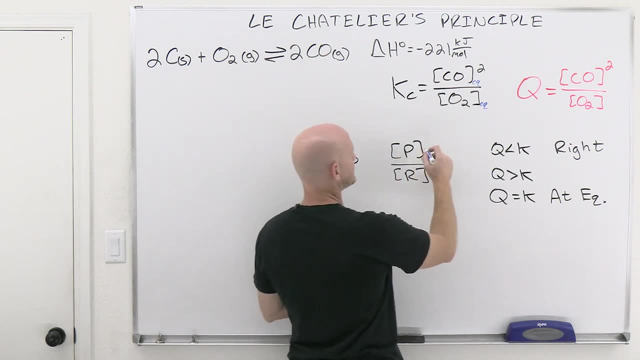 go smaller and smaller and smaller until the end of the reaction, right when it equals K, And so when Q is bigger than K, that ratio needs to come down, And to come down we're going to have to convert some products into reactants in this case. So 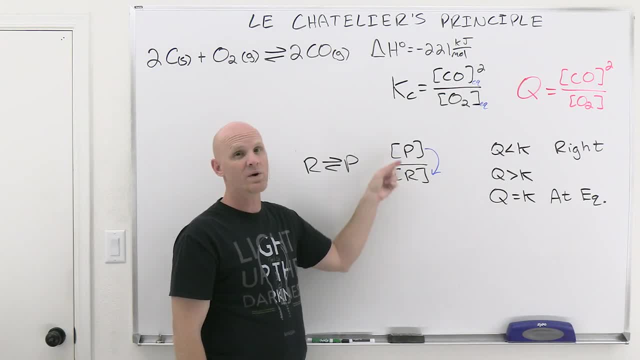 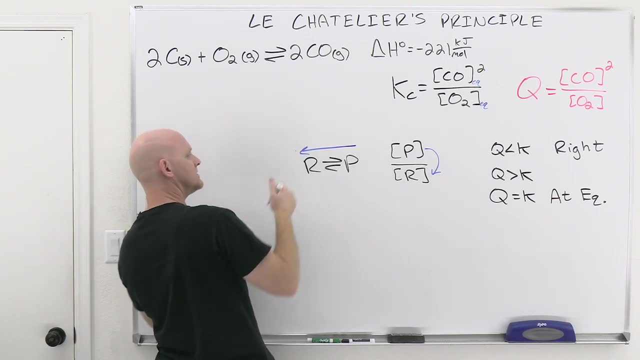 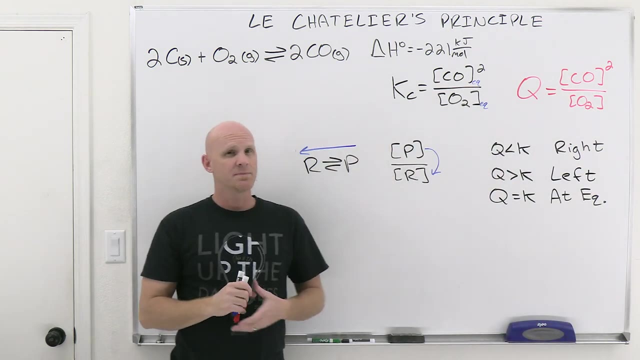 we need to make the numerator smaller and the denominator bigger, so that overall, this ratio is going to decrease. Well, to turn products into reactants, we refer to that as the equilibrium shifting to the left instead, And so now we've got a great little comparison, If at any point in time, I know the concentrations. 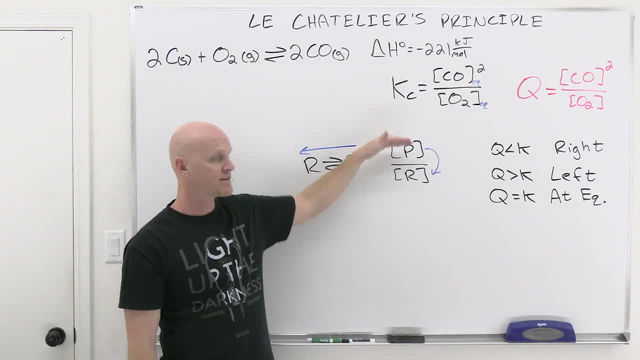 of all reactants and all products, and I measure them. I can look at that ratio of products to reactants And I can look at that ratio of products to reactants, and I can look at that ratio of products to reactants. And is it equal to K? Well then, I've already reached. 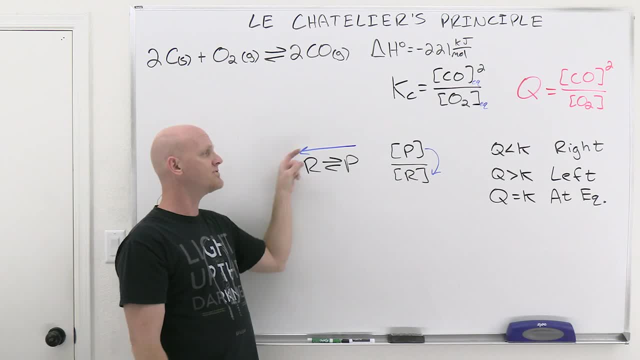 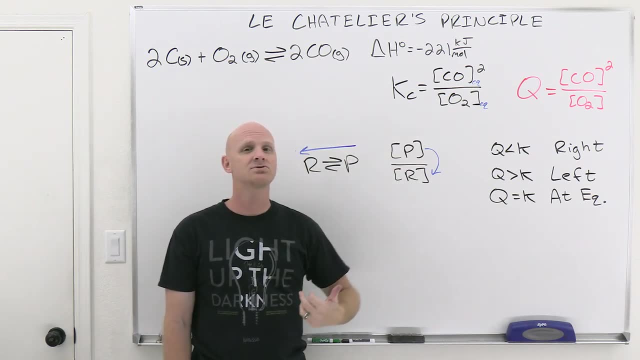 equilibrium. But if it's smaller than K, that reaction needs to go in the forward direction and proceed to the right. But if Q is bigger than K, the reaction actually needs to go in the backward direction and proceed to the left. And so now we've got a really good test to figure. 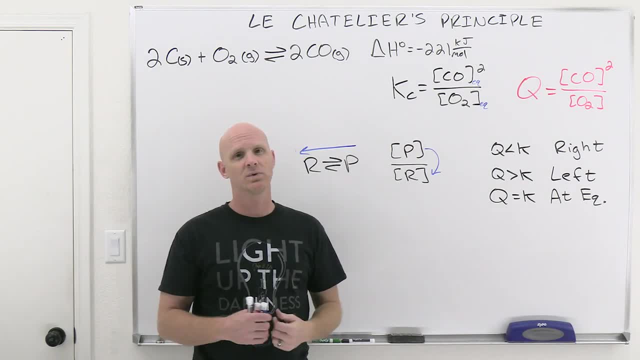 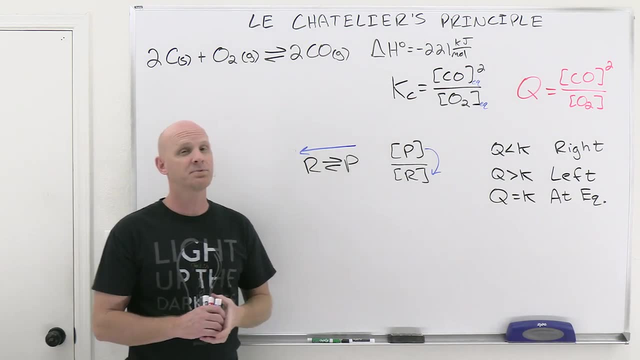 out which way a reaction needs to go. if it needs to go anywhere to get to equilibrium, Cool, And that's one way we can look at Le Chatelier's principle. Another way it turns out we can look is just simply by looking at the definition. If you place a stress on a 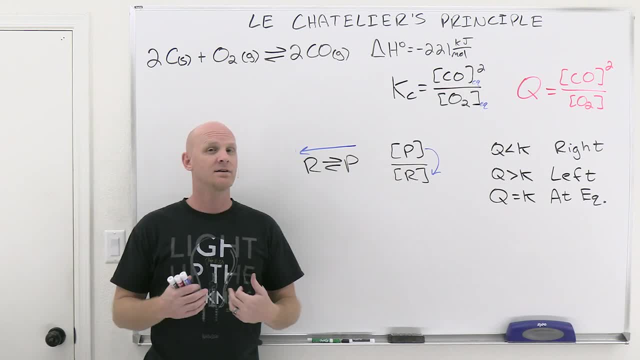 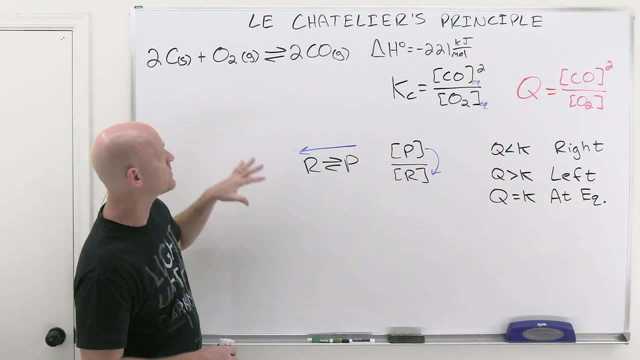 system. you can look at the definition of stress And if you place a stress on a system, you can at equilibrium, the system will react, or I should say the system will counteract that stress to get back to being at equilibrium. That's Le Chatelier's principle. So that'll be another. 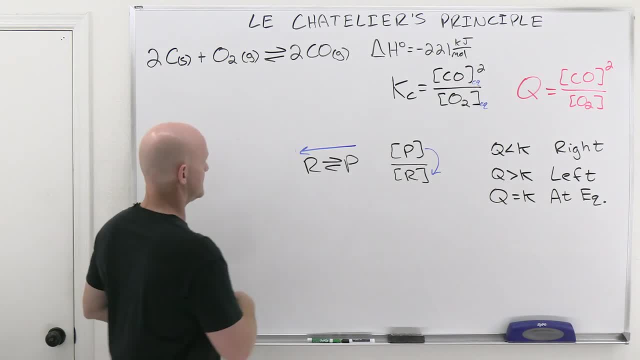 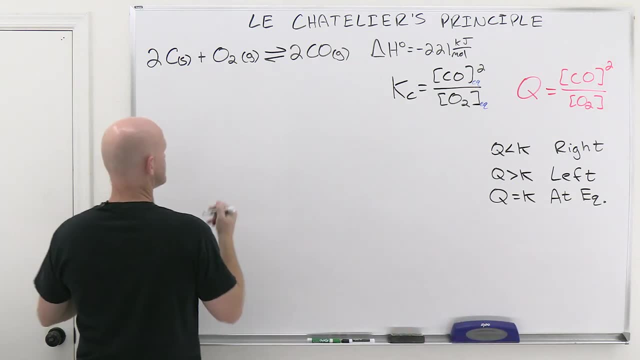 way we can look at it, And so we're going to take a look at a few different things here. but we're definitely going to need some room, And so we're going to look at some stresses, or at least potential stresses, and see what effect they're going to have, And so 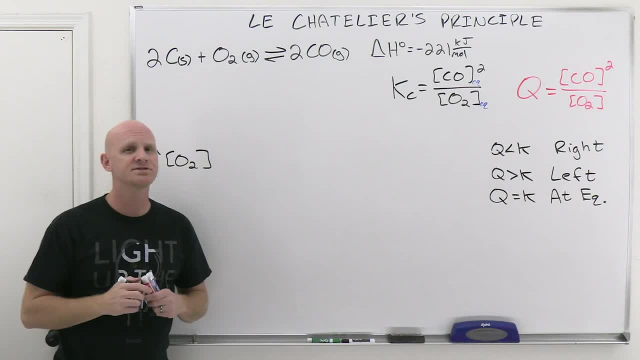 the first stress we're going to look at is increasing the concentration of O2.. Now The first thing we'd ask ourselves: is it a stress? And a stress again is defined as anything that takes the system out of equilibrium, that removes it from equilibrium. 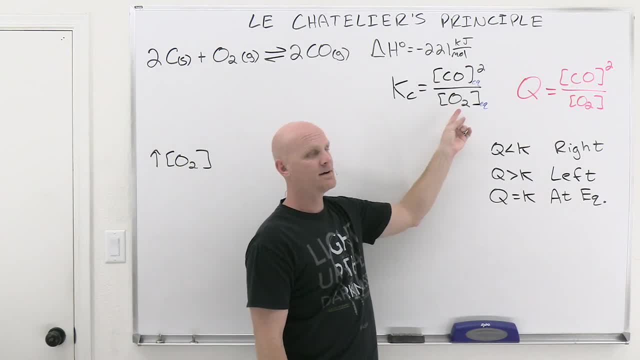 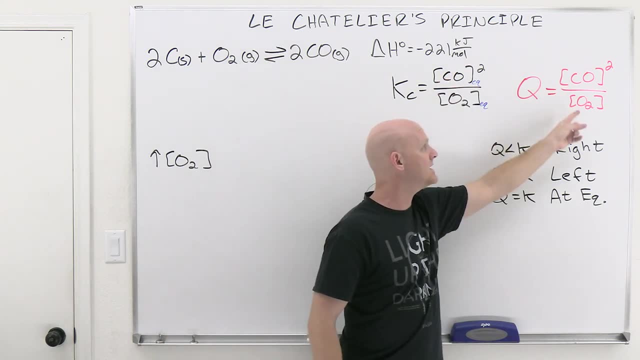 Well, in this case, by adding O2, I change the ratio. And so, again, if the system is already at equilibrium to begin with, then this ratio right now equals K and it equals Q. By adding O2, it changes the ratio, which means it's no longer equal to K. 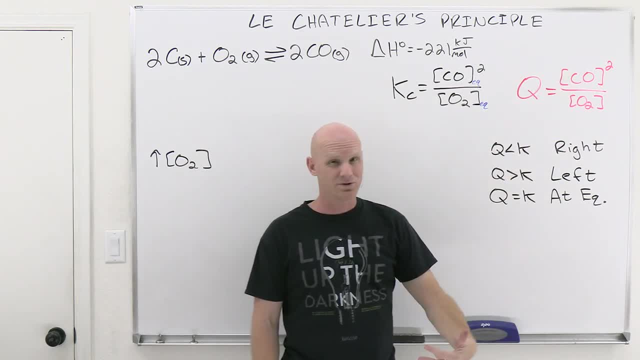 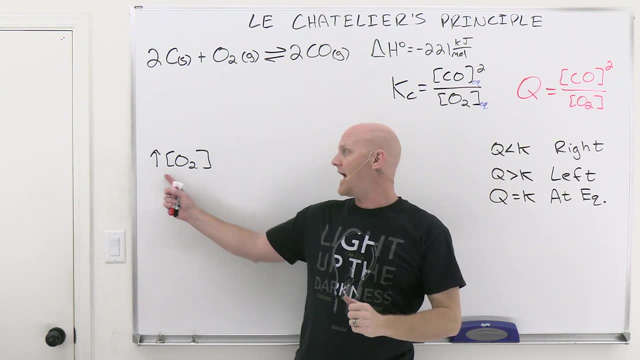 This no longer applies, but it's still equal to Q. It's just a new Q value, The Q changed. So again, when you're not at equilibrium, this ratio only equals Q. It does not equal K. Well, by adding O2, what did that actually do to this ratio? 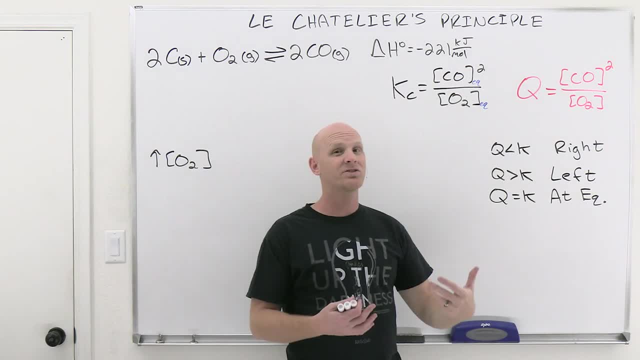 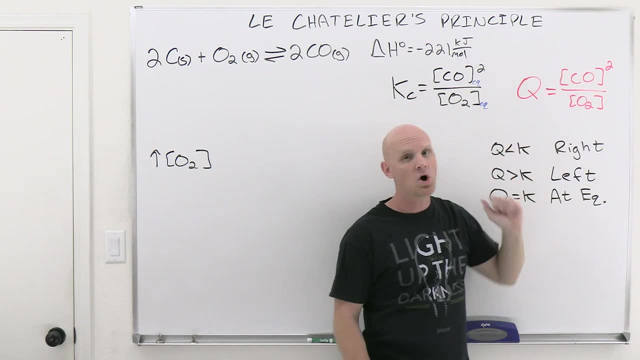 Did it make it bigger or did it make it smaller? Because a second ago it was actually equal to K. Well, in this case, by increasing the value of the denominator, it makes this ratio smaller. So let's kind of take a look at this graphically. for a second, 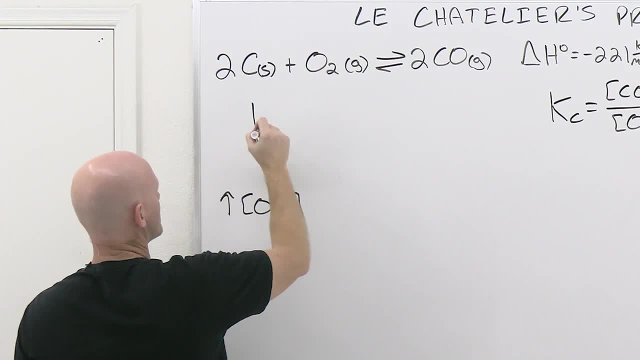 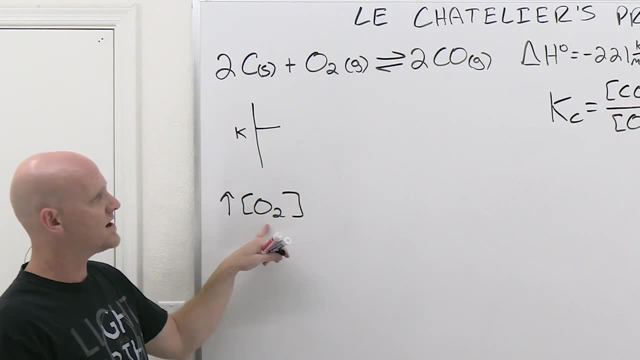 And so we're going to have a reaction, And what we're going to have is K right here And when I increase the concentration of O2.. So, and actually I guess we should look at this as Q, but this value right here specifically, is K. 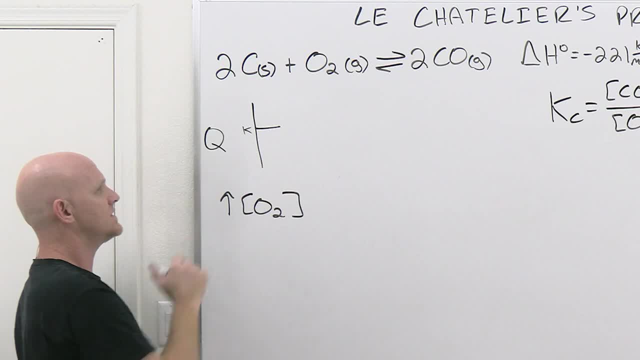 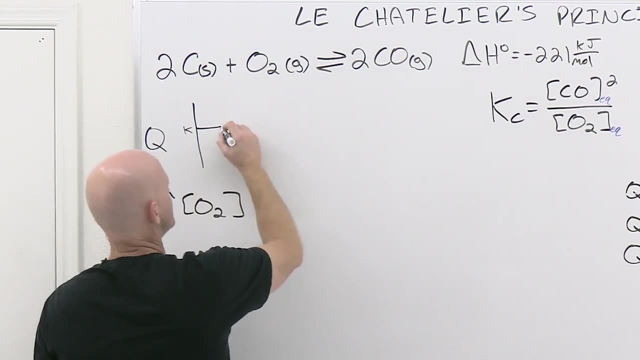 And so it starts out: it's at equilibrium, And at some point in time we're going to increase the concentration of O2. And by increasing the value of the denominator it's going to make the overall ratio smaller. And so all of a sudden, that value just went down. 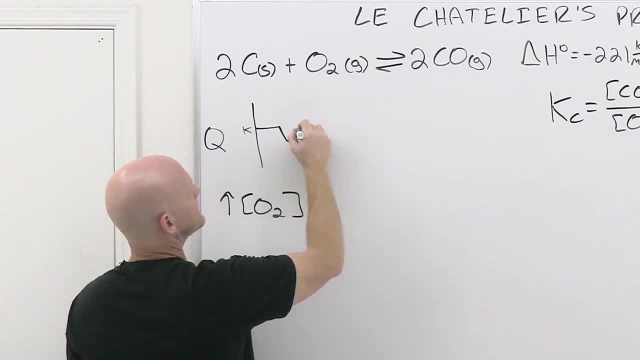 And what you're going to find is that this value is going to gradually increase to get back to being equal, So it's going to be less than or equal to K, And so at this point, right here, we've got Q less than K. 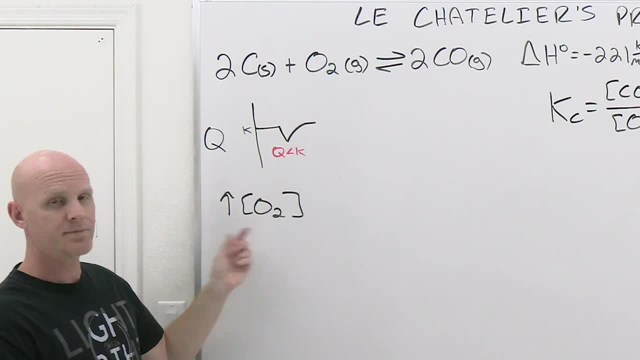 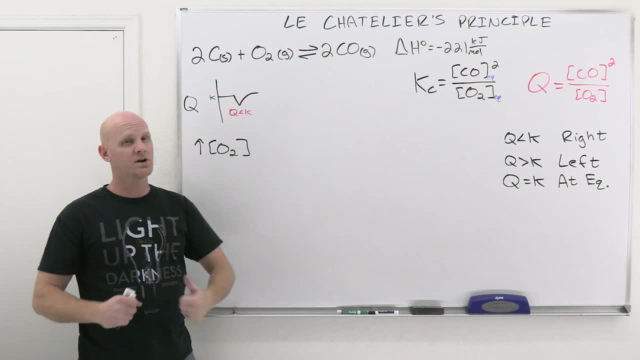 And because Q is less than the K value, because that stress we put on it right there, the equilibrium needs to shift to the right, to get back to being at equilibrium. So that's one way to look at this. You figure out okay what we did. 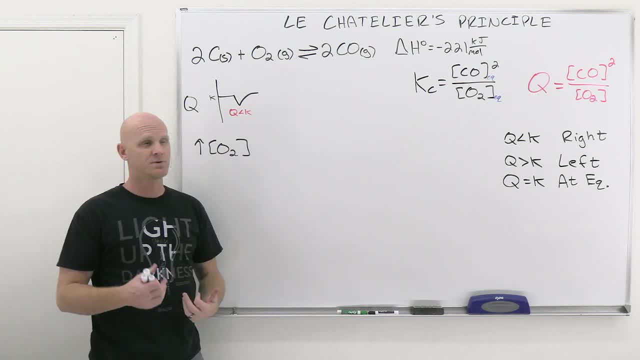 How did it affect Q? Did it make Q bigger than K or smaller than K? Or did it even change the value of Q? And in our case it made Q less than K. so it's got to shift right. One way to look at it. 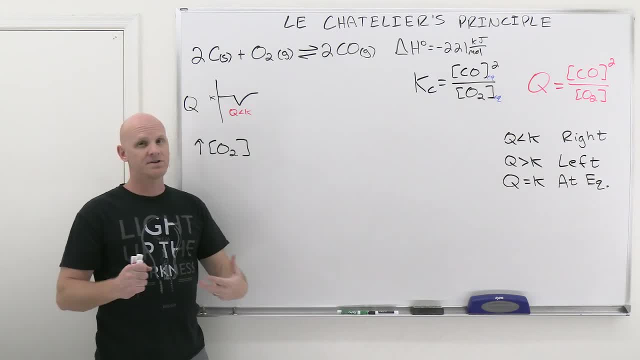 The second way is using Le Chatelier's principles of the definition. If you place a stress on a system at equilibrium, it will respond to counteract the stress. Well, in this case, the stress is that we added O2.. It definitely took the system out of equilibrium. 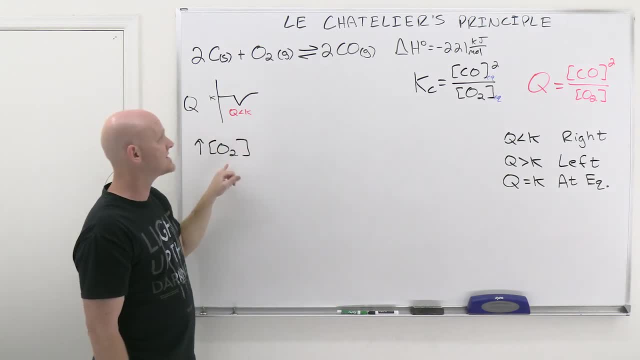 because it changed that ratio And the stress is that now we have too much O2.. Well, you only got two options: You can either shift right, or you can shift left, Or I guess you can not shift at all. if it's not a stress, it turns out. 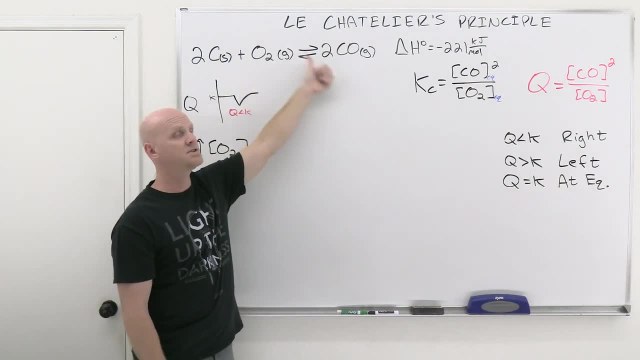 But in this case it is a stress. So, shifting right, shifting left, Which one counteracts the stress? Well, the stress is that we have too much O2.. If I shift right, it uses up the O2.. If I shift left, it makes even more O2.. 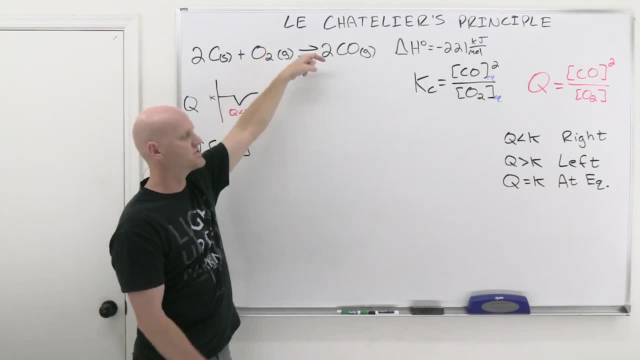 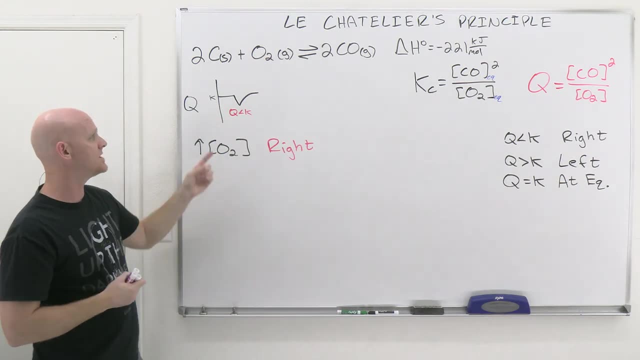 Well, which one's counteracting? the fact that we have too much Shifting to the right. Cool, And shifting to the right is going to cause your Q value to go up, So as you convert reactants into products until it's back to being equal to K. 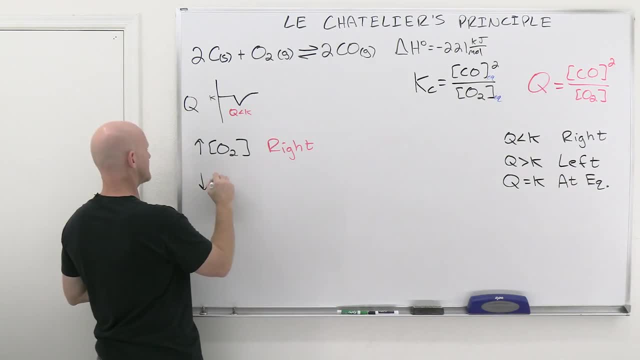 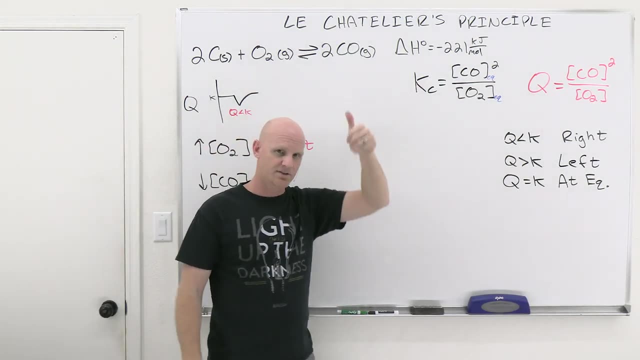 All right. So the next stress, or potential stress we'll look at is decreasing the concentration of carbon monoxide, And the first question is: is it a stress? Does it change the ratio? Yes, Then it's going to take the system out of equilibrium. 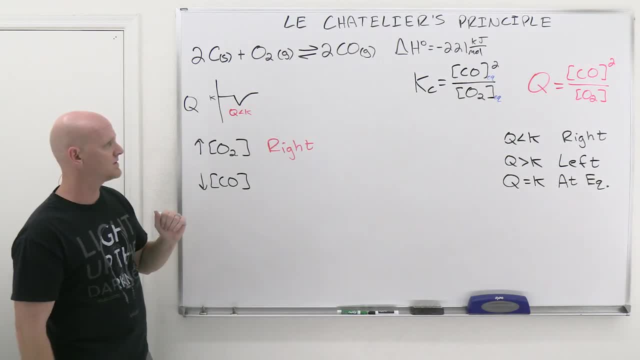 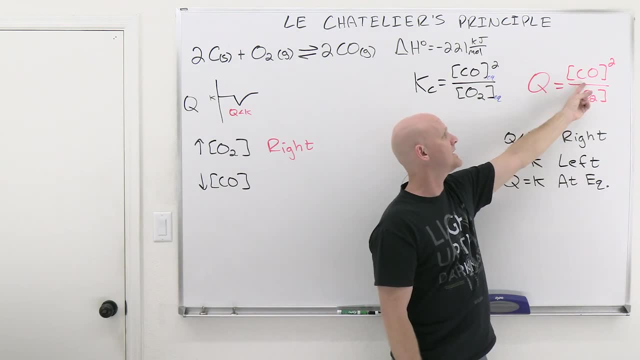 And we're definitely going to classify this as a stress. Now, in this case again, since we changed this concentration, this ratio no longer equals K, it just equals Q, And by lowering the concentration which is in the numerator, so lowering the concentration of a product. 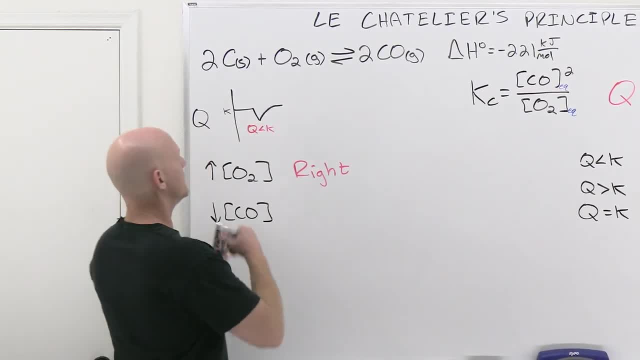 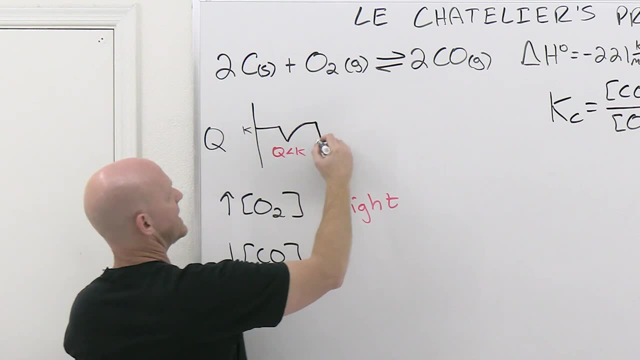 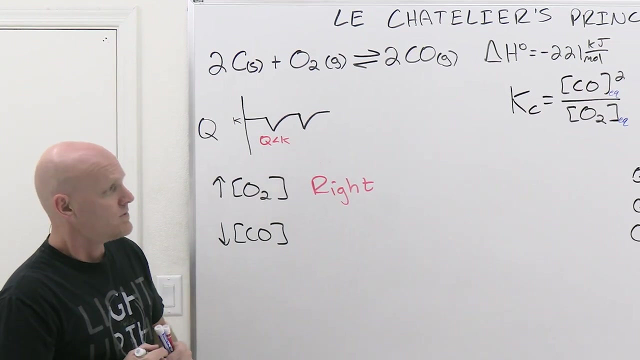 it lowers the overall ratio. So once again, we just did something that's going to cause our ratio to go down And it's going to counteract that stress by trying to increase until it gets back to being at equilibrium. Okay, Now again the other way to look at this. 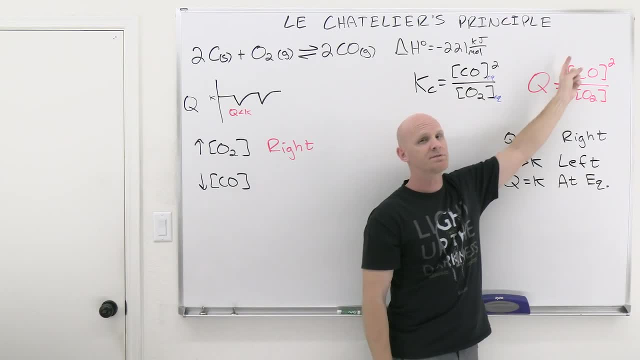 again in terms of Q and K, is that by lowering his concentration, we've lowered the value of the ratio? A minute ago, that ratio was equal to K. When Q is equal to K, it was at equilibrium. Since we lowered the ratio, 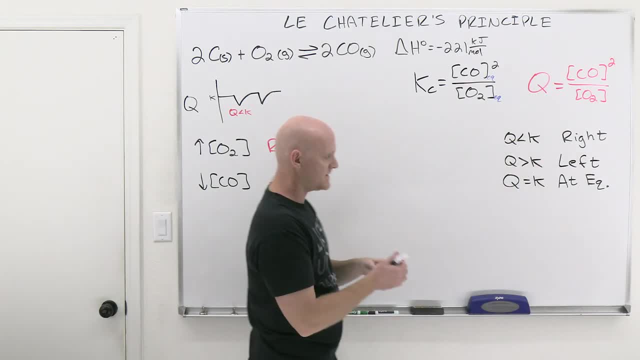 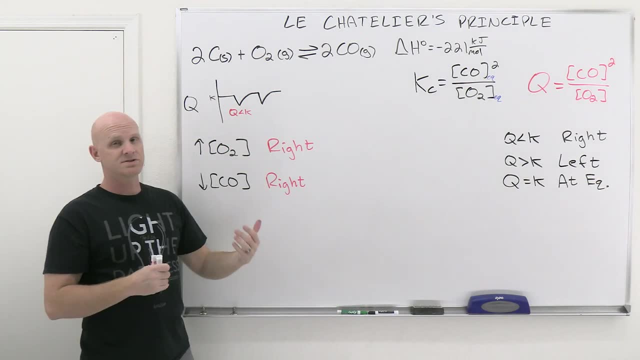 Q is now less than K Again, and the equilibrium needs to shift to the right to get back to equilibrium. So and again, if we use Le Chatelet's definition, the stress is that we've lowered the concentration of CO. 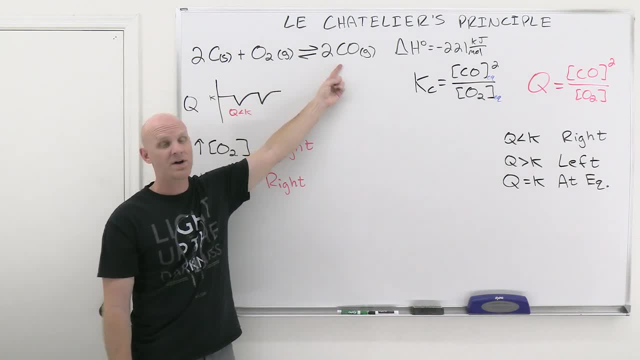 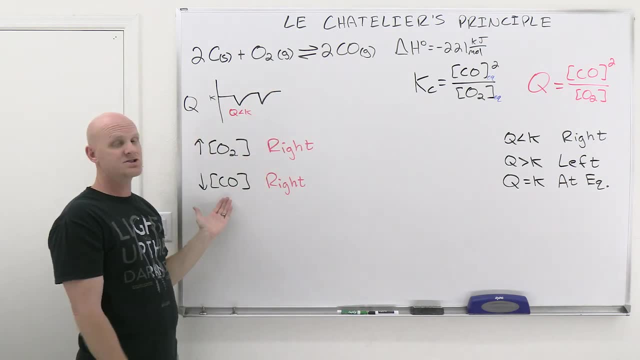 It means there's no longer enough CO to be at equilibrium. We don't have enough. So if I shift to the right, I'll make some more. If I shift to the left, I'll use up what I have, Which one counteracts the stress of not having enough. 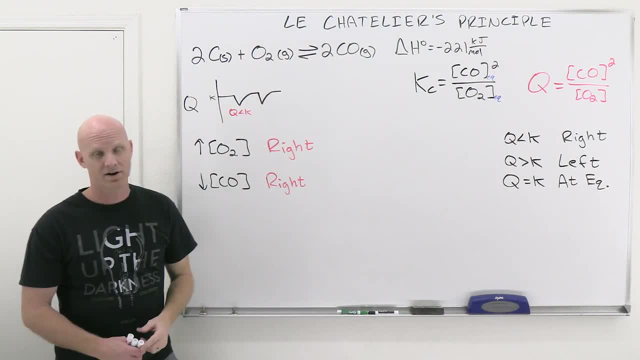 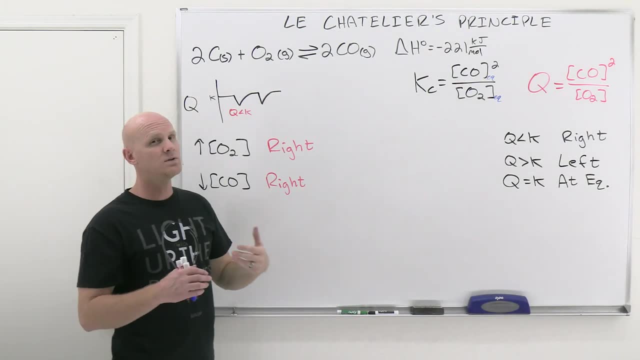 Shifting to the right to make more. So that's how we kind of use the definition there. Now it turns out one other way to look at this is from a kinetics perspective. So in the last lesson we said that equilibrium, dynamic equilibrium, chemistry. 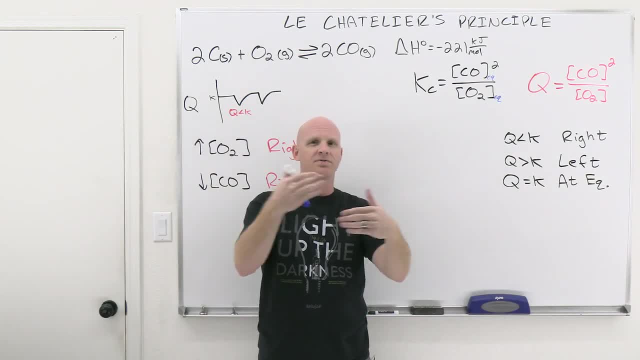 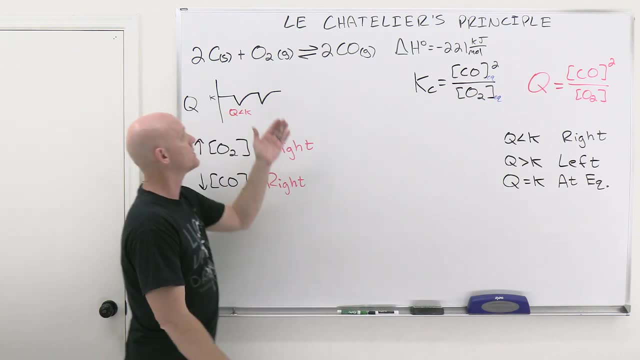 means that the forward rate equals the reverse rate. The rates are proceeding at the same rate. We learned from rate laws in the last chapter that rates typically depend on concentrations of reactants, And so the forward rate is going to depend on how much reactants we have. 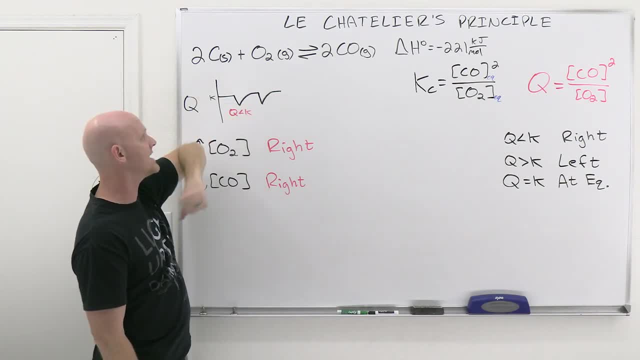 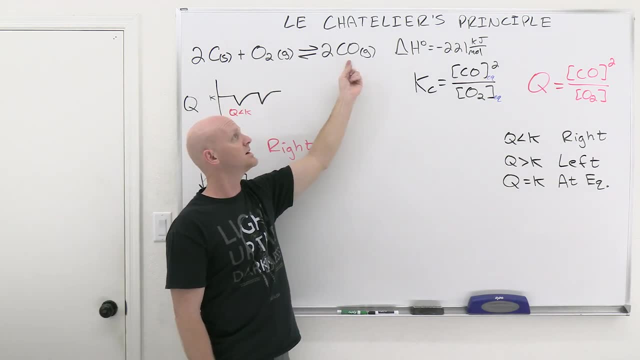 In this case, solids. usually, well, I guess solids can affect rates, but we're going to focus on the gas here, So the forward rate is going to depend on how much O2 we have. The reverse rate, though, is going to be dependent upon how much CO we have. 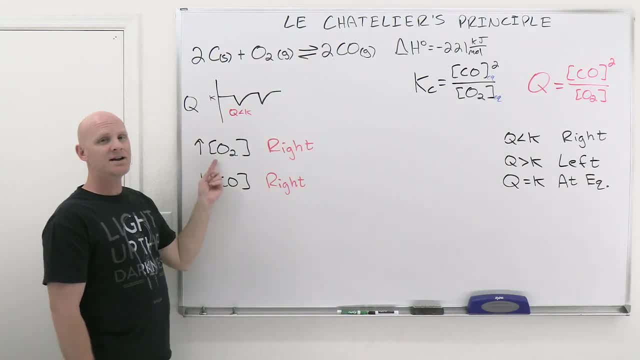 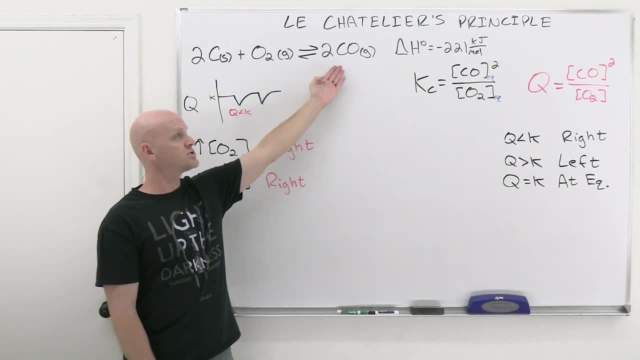 the reactant of the reverse reaction. And so when we added O2, it added the amount of reactants we had that were doing the forward reaction, and so it sped up the forward reaction. The reverse reaction for that split second remained unchanged. 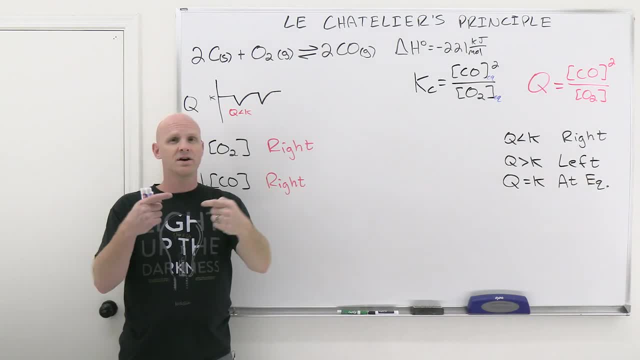 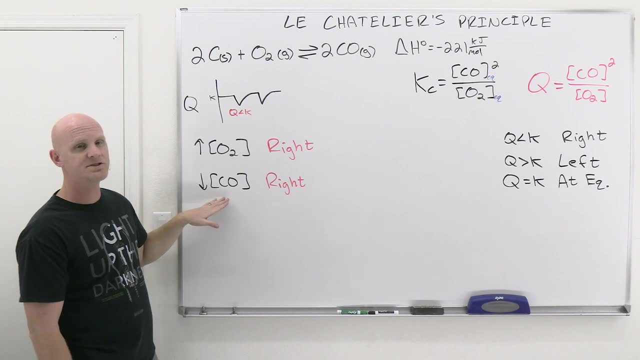 but the forward reaction just got faster. So if they were equal a second ago, well now the forward reaction was faster and the reaction overall was proceeding to the right. In the second case we lowered the concentration of CO. Again the rates were equal. 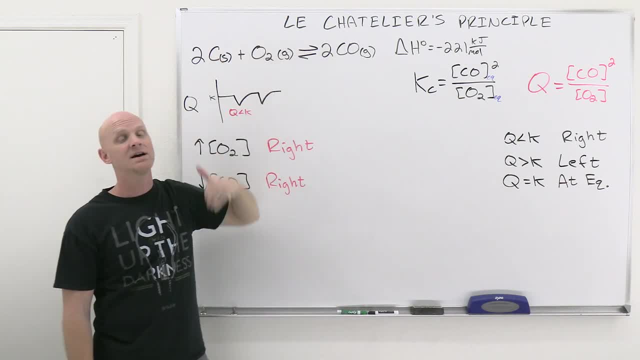 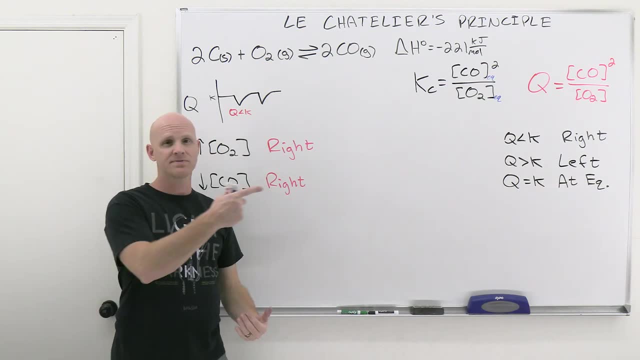 but now we lowered the amount of the reactant for the reverse reaction. It slowed down the reverse reaction And so if a minute ago the rates were equal, well now, because I slowed down the reverse reaction, the forward reaction is faster again. 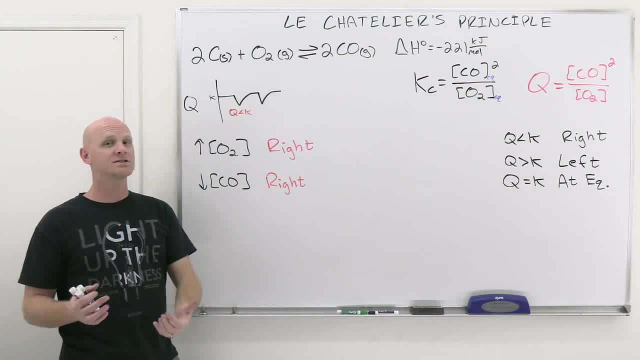 and overall that means it's proceeding to the right And that's how we kind of look at this from a kinetics perspective. But whether you look at Q versus K or just the definition of Le Chatelier's principle from a conceptual perspective or the kinetics perspective, 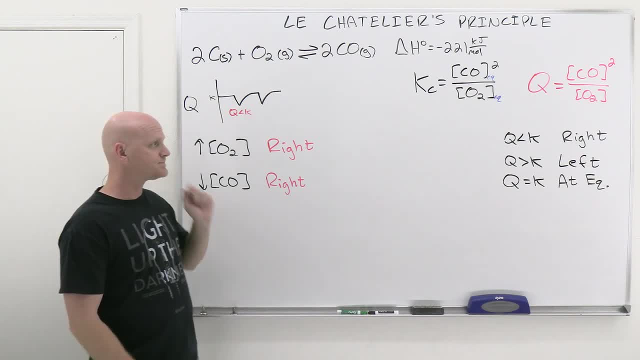 they should always lead you to the same conclusion. Okay, so now we want to take a look at an important exception that you should realize, And we're going to add or remove a solid, And you might recall that solids and liquids typically don't show up. 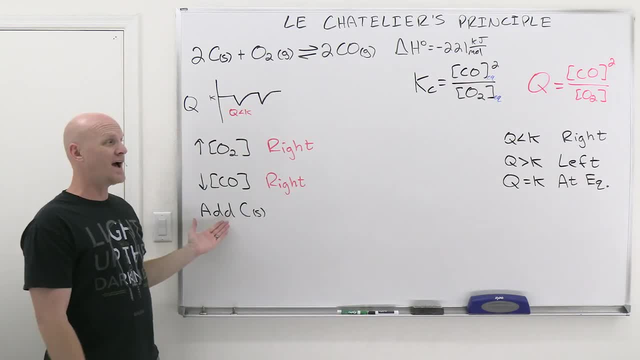 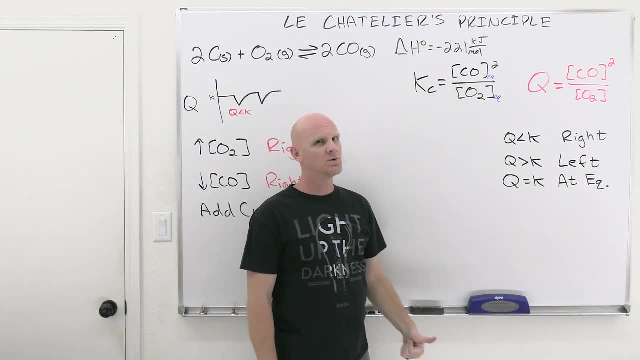 in the equilibrium constant expressions, And so when you add one, it doesn't actually change your ratio. And if it doesn't change your ratio, then you're still at equilibrium. And if you're still at equilibrium, Q equals K and there's no shift. 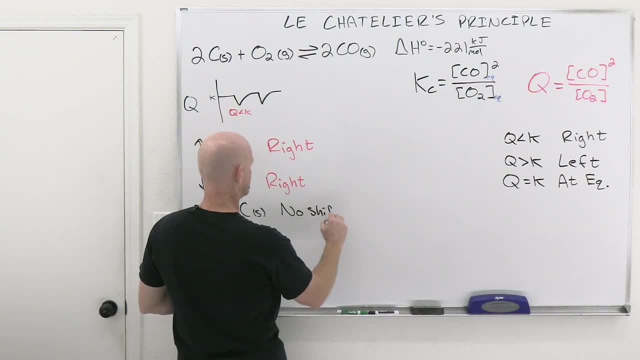 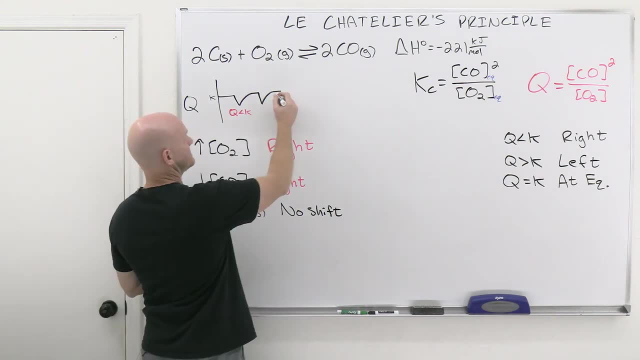 And so adding a solid here or removing a solid will result in no shift in the equilibrium: Not left, not right, no shift whatsoever, because you're still at equilibrium. And so in this case, when we add the carbon solid, it doesn't take the system out of equilibrium. 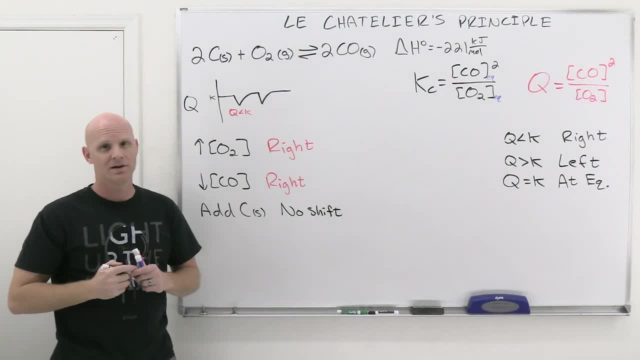 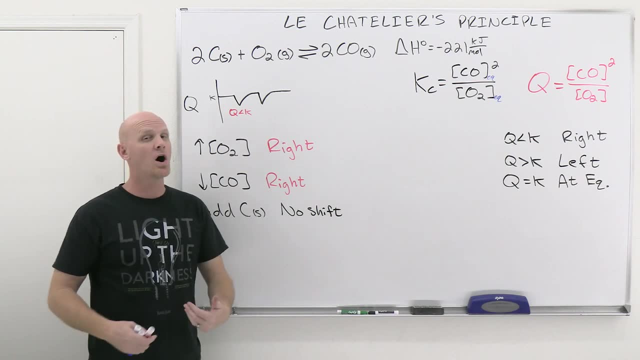 and therefore Le Chatelier would not consider this a stress. Now, be careful here, because solids can be affected by a shift, but they can't cause one. So we see here that adding our solid here doesn't shift it one way or the other. 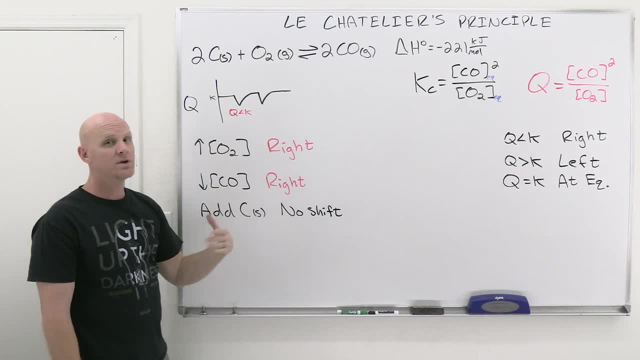 However, when we had shifts up here, it would affect the amount of solid present in our container. So in this case, both of these were shifting to the right and, as you shifted to the right in these first two examples, that's going to use up carbon solid. 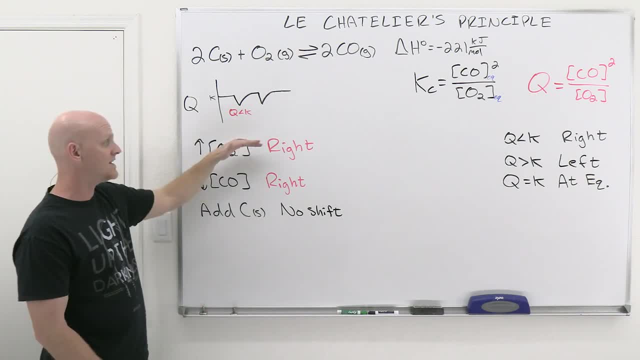 We're going to end up in a situation where there's less carbon solid in our container, And so anything that can cause a shift will affect the amount of solid in your container. So, however, if you yourself add or remove the solid from your container, 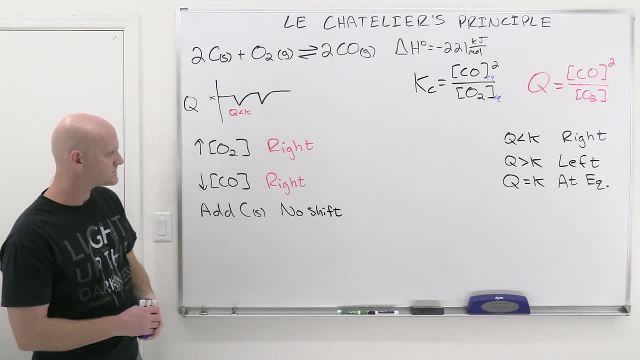 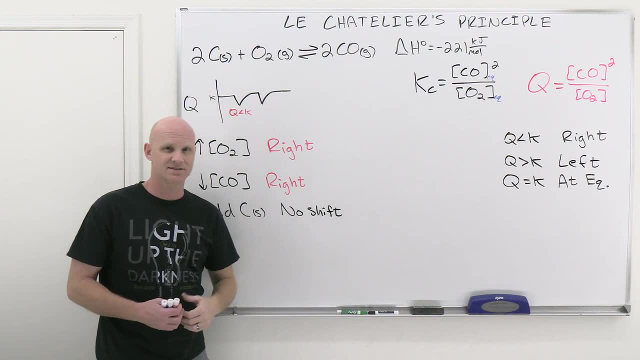 it itself will not cause a shift. Okay, so keep that in mind. Next thing we want to look at are the trickiest ones of all, and that's temperature and pressure effects. Students get a little tripped up on these, especially this temperature one. 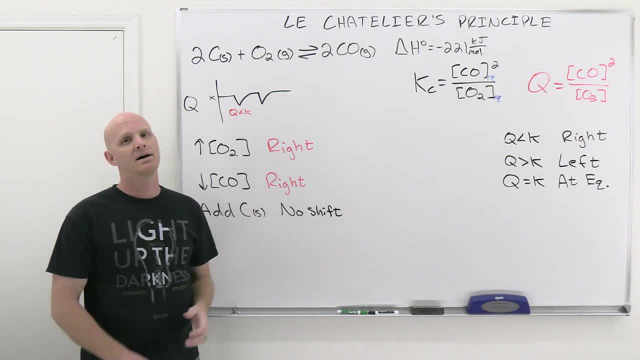 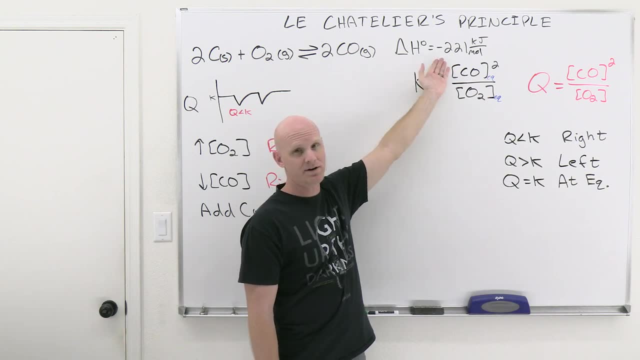 as we'll see- And temperature effects. to be able to evaluate those which way they're going to cause a shift, you have to know if the reaction's endo or exothermic, And that's why I put delta H up here. 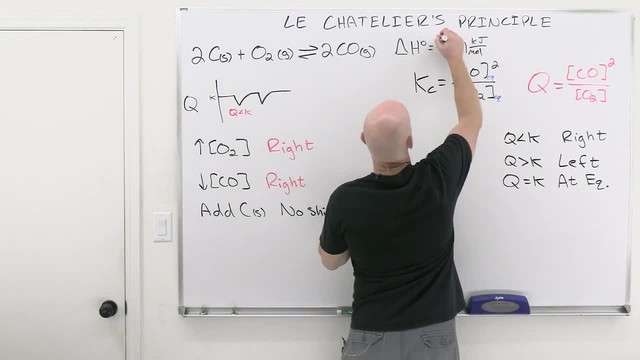 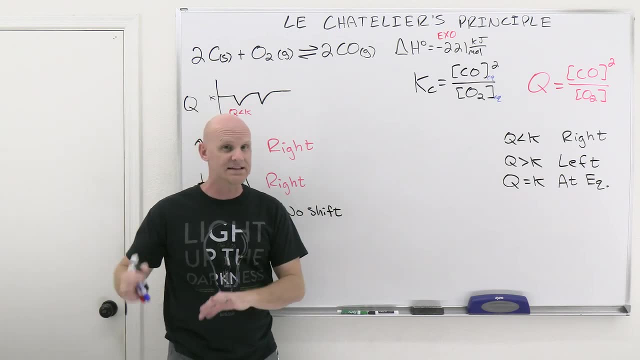 Delta H is a negative number, and a negative number means it is an exothermic reaction. In an exothermic reaction, the hallmark is that it gives off heat, It releases heat, It produces heat. ie, heat is a product. 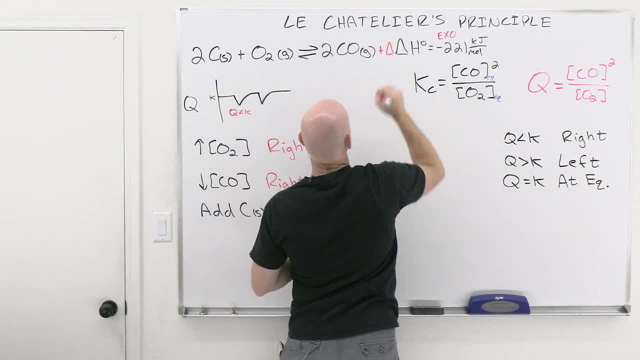 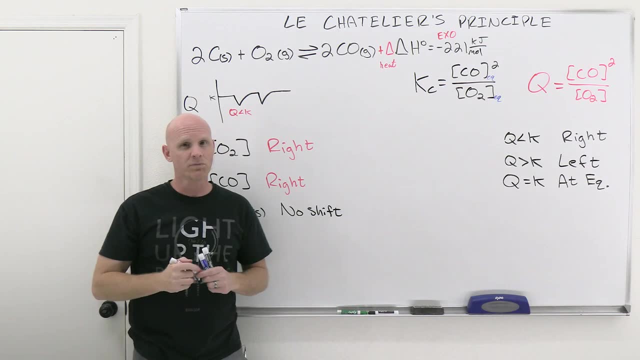 And so we can write heat over here, and commonly heat is symbolized by the delta symbol. I could have just simply put plus heat as well. same diff. But the key is I only knew to put heat on the product side because it was an exothermic reaction. 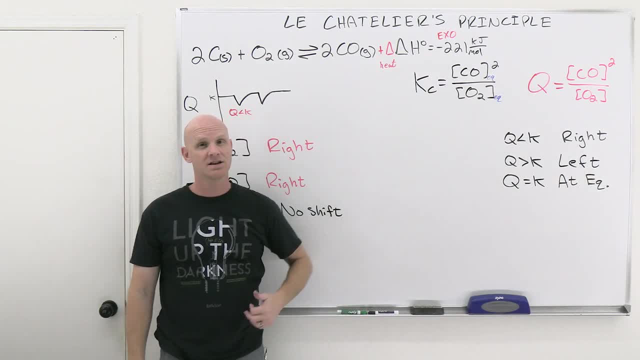 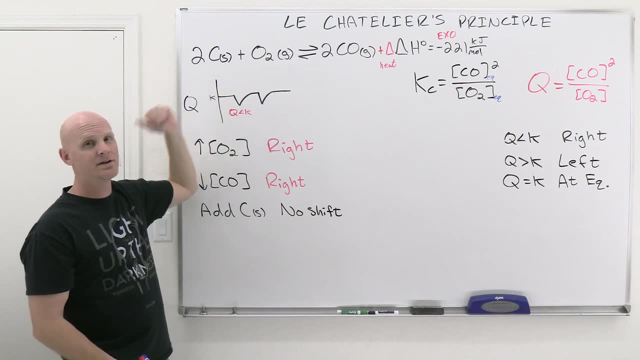 since delta H was negative. Had I given you delta H being a positive number, well then I would have had to realize that that reaction uses up heat, it consumes heat and heat's a reactant, and I would have had to written it in over here. 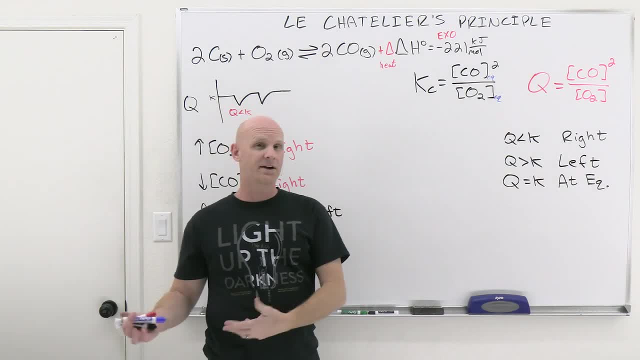 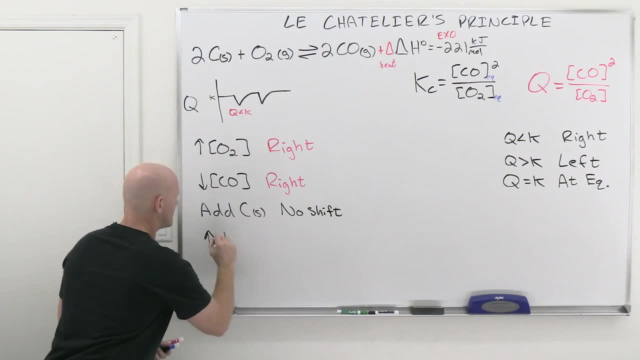 And so whether it's endo or exothermic will determine on whether heat is a reactant or a product, Whether you raise the temperature or lower the temperature- and in our case we're going to raise the temperature- that's going to be determining. 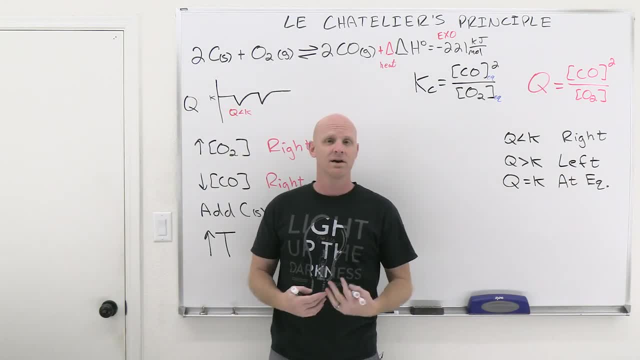 whether or not you add heat or remove heat. When you raise the temperature, you're adding heat. When you're lowering the temperature, you're removing heat. And so when you see raised temperature, you should know: oh, that means the same thing as adding heat. 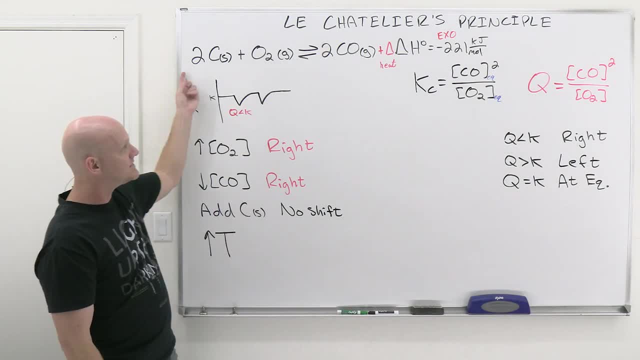 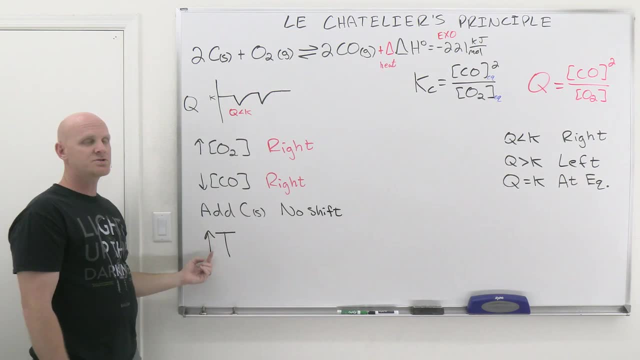 What you need to figure out, though, am I adding a reactant or adding a product, based on if it's endo or exothermic, And so, in this case, being exothermic, heat is a product. Raising the temperature, then, for this reaction right now. 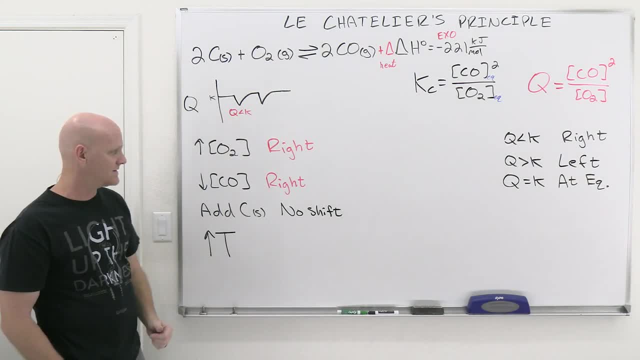 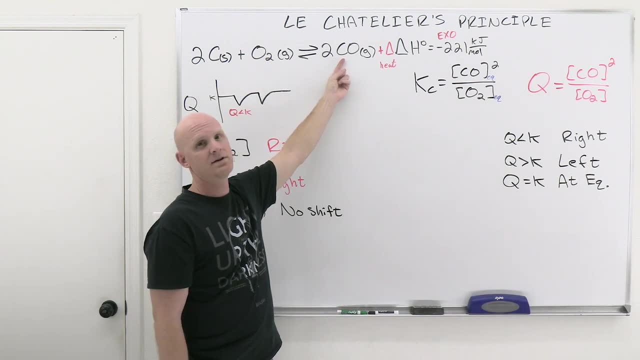 means adding a product, not adding a reactant, And so in this case, it's going to do the same thing as if we just added any other product as well. If we'd added CO instead, it would have resulted in a shift to the left. 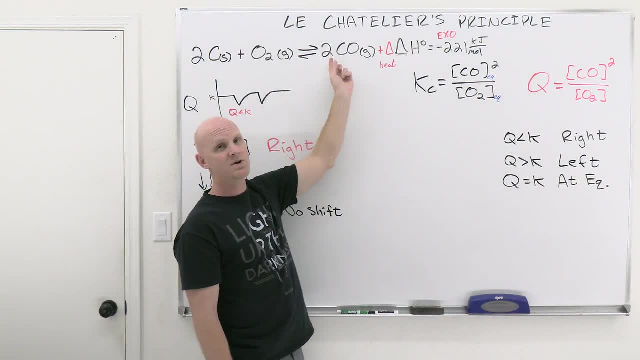 Notice when we remove CO, it shifted right. If we add CO, the stress is too much CO and we need a shift left to use some of it up. So adding a product here would have resulted in a shift left. Well, adding heat when heat's a product. 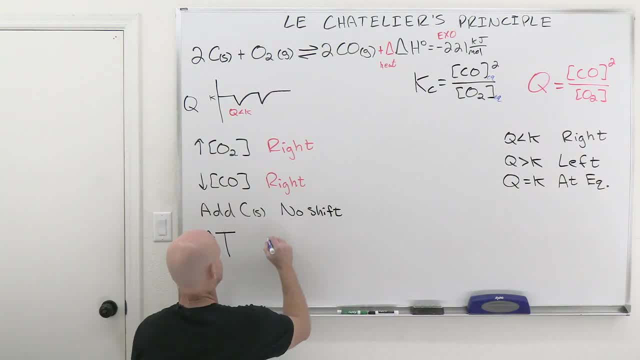 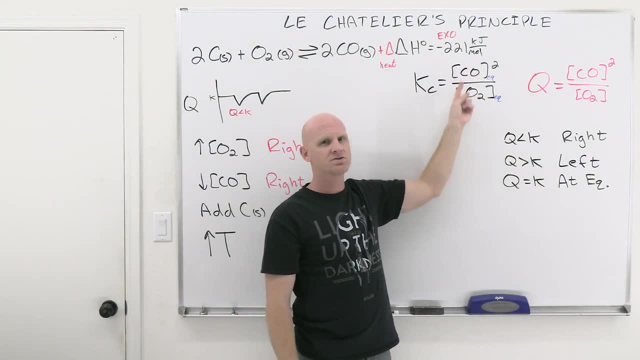 is also going to result in a shift to the left. But this one's tricky because if you look by adding heat, did I change this ratio at all? Well, I didn't. Then you might be like: well then, we're still at equilibrium. 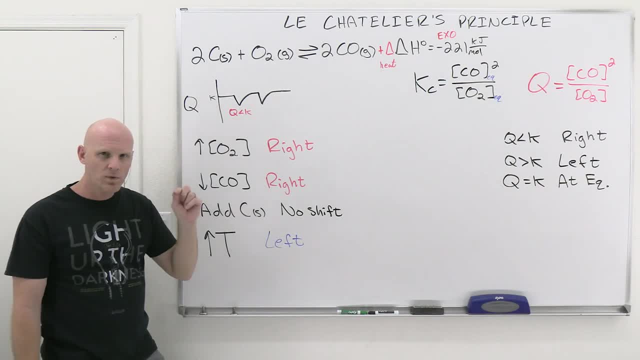 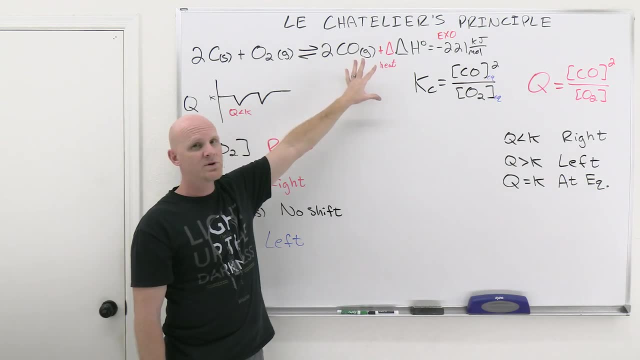 Well, we're not Because, if you recall, temperature is the only thing that actually changes the value of the equilibrium constant And in this case, if whatever you do with temperature causes a shift to the left, like it is in our case, 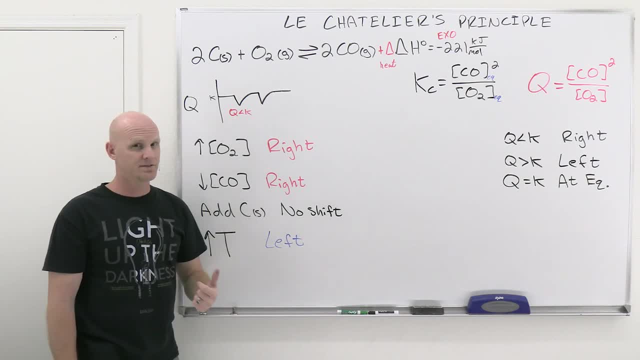 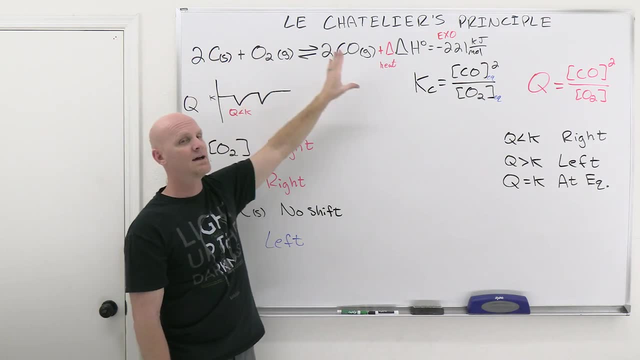 well, that means when you you're going to establish a new value for the equilibrium constant first off, when you change the temperature And if you shift left, you're going to end up in a situation where you have more reactants and less products. 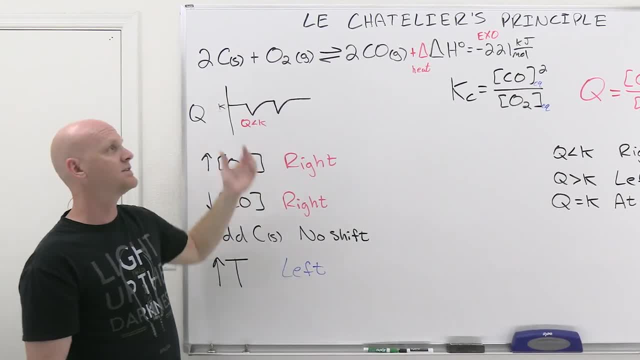 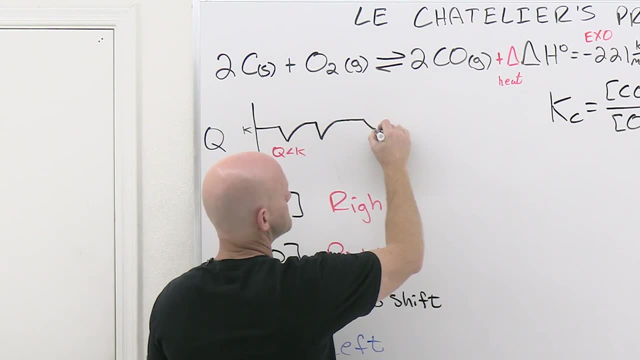 than the old equilibrium constant, And so more reactants, less products, that's a lower value to the equilibrium constant. And so what we're going to find is that we've just established a new equilibrium constant for this new temperature, this higher temperature. 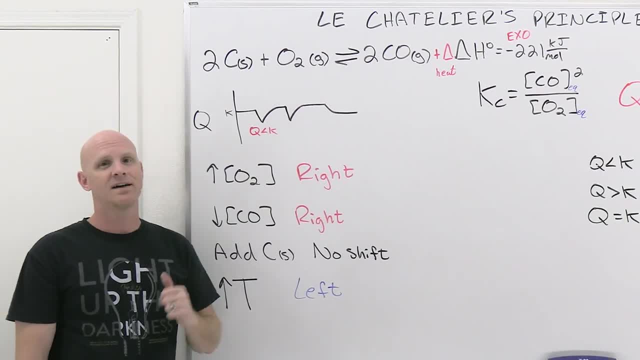 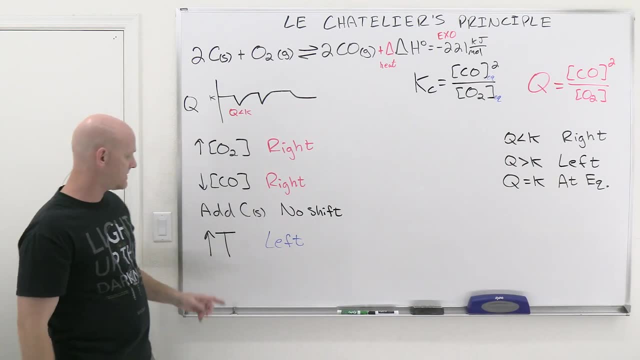 And so, whatever you do with temperature, if it shifts left, that's going to be a new lower equilibrium constant value. If it shifts right, that would be a new higher equilibrium constant value. So if, instead of raising the temperature for this exothermic reaction, 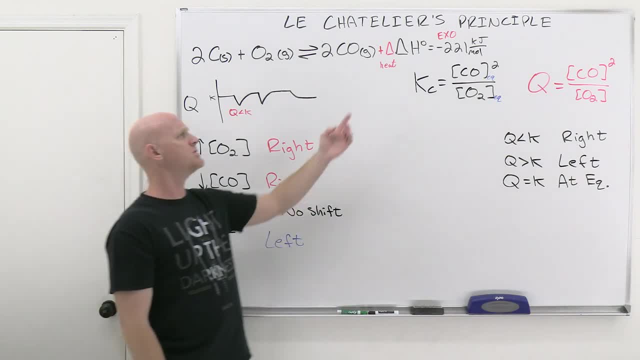 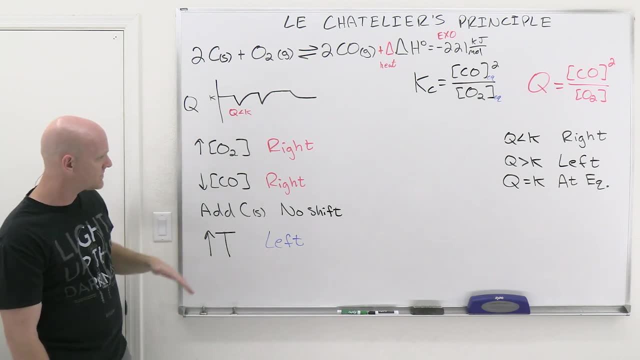 we had lowered the temperature. well, lowering the temperature would have been removing heat and we would have needed to make more, And shifting to the right with temperature raises the value of the equilibrium constant. So notice all the other changes we've done so far. 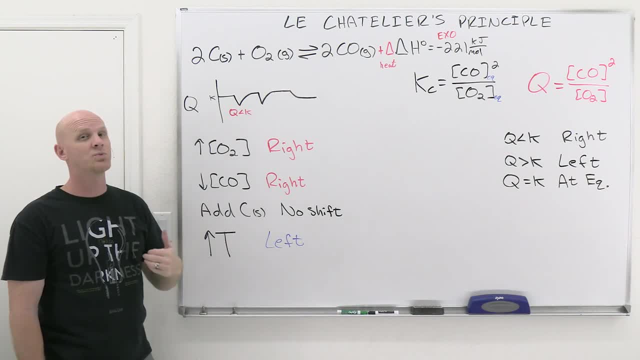 never changed the equilibrium constant, It just changed the reaction value. It changed the reaction quotient, Q, And then we had to strive to get back to being at equilibrium. But temperature is the one thing that doesn't change your Q, it changes your K. 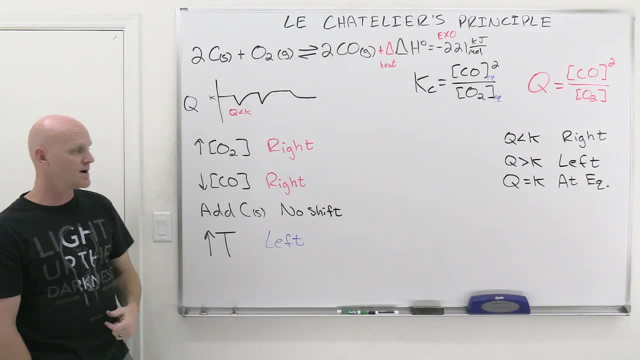 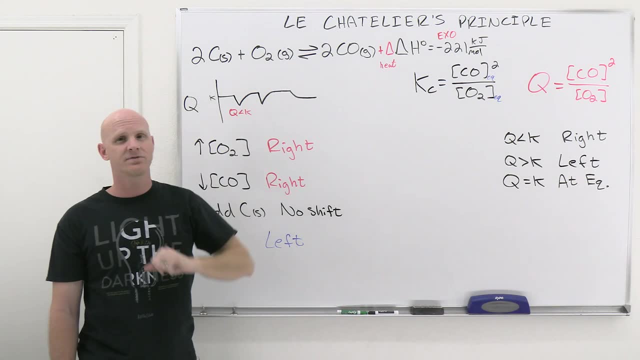 And Q has to shift to equal the new equilibrium constant. All right, so that's temperature effects. It's super tricky. You've got to know which side is heat on, based on if it's endo or exothermic, And then you've got to know 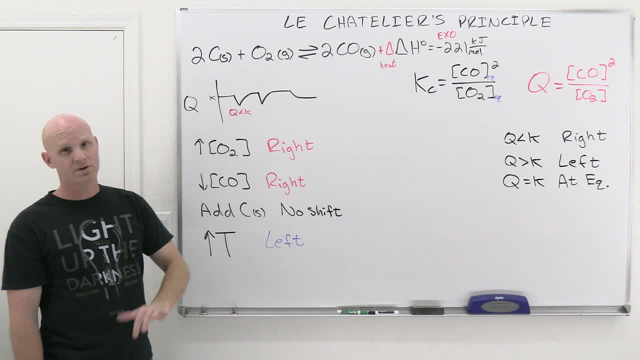 are you adding heat or removing heat, based on if you're increasing the temperature or decreasing the temperature? And then sometimes you might have to know: did that make K bigger or make K smaller? And again, with whatever you do with temperature shifts, left. 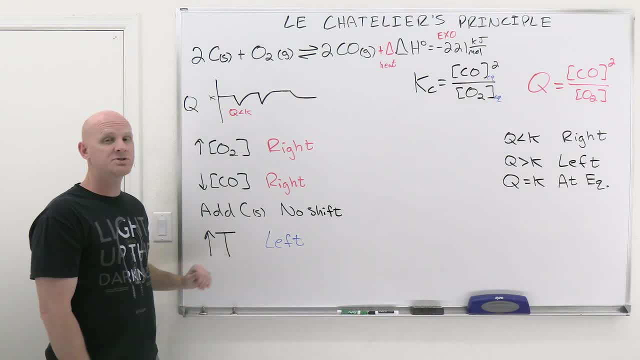 K is now smaller. If whatever you do with temperature causes a shift to the right, K is now going to be bigger instead. All right, so pressure effects. So pressure effects are going to be tricky here, And so we're going to increase the pressure. 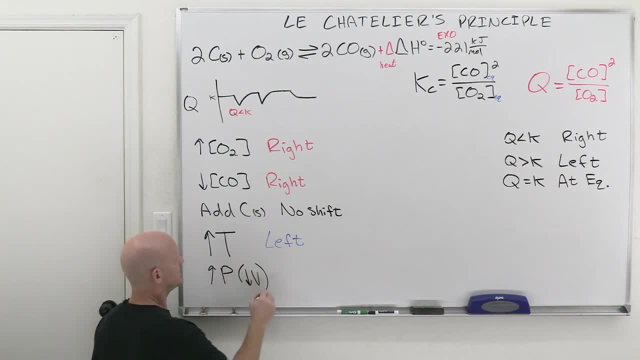 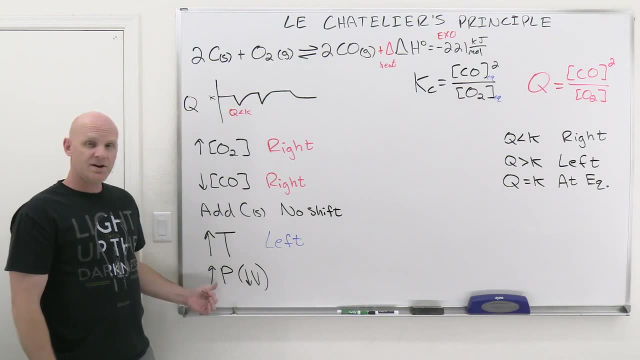 And we're going to increase the pressure by decreasing the volume of the overall container, And that's where things are going to get a little bit tricky. So easiest way to increase pressure- And so you're going to treat these as synonymous- We're going to increase the pressure. 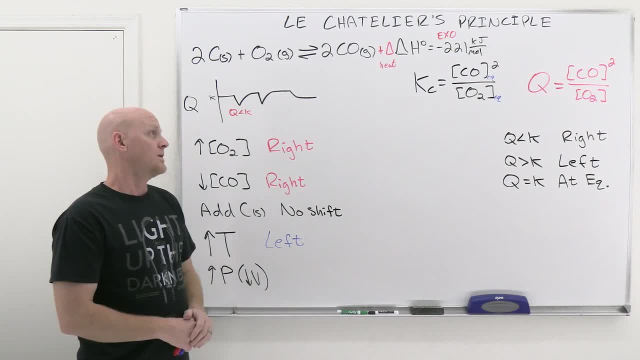 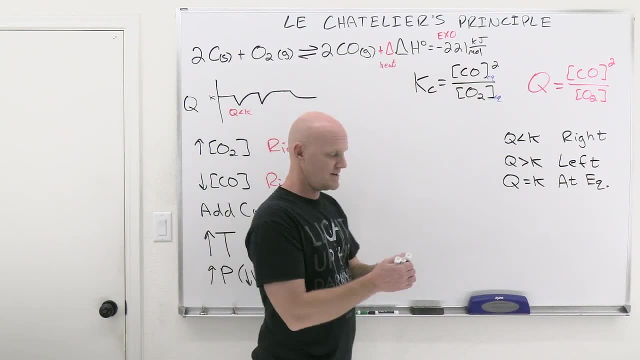 by decreasing the volume. Cool now you might be like: well, Chad pressure doesn't show up here. Well, but volume does, because these brackets mean molarity And, if you remember, molarity equals moles over the volume in liters. 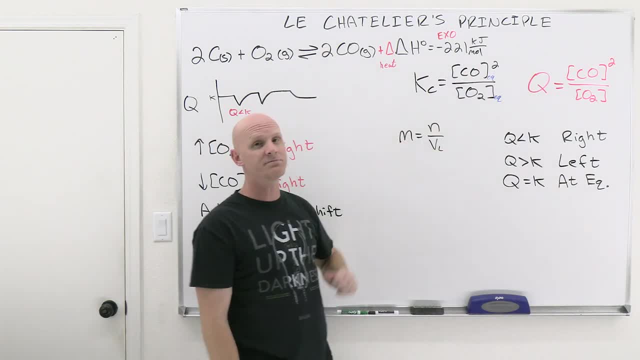 And so, even though you don't see volume up here, it's implied as part of molarity. And notice: you have molarity squared in the numerator, but you only have molarity in the denominator, And so part of this is not actually going to cancel. 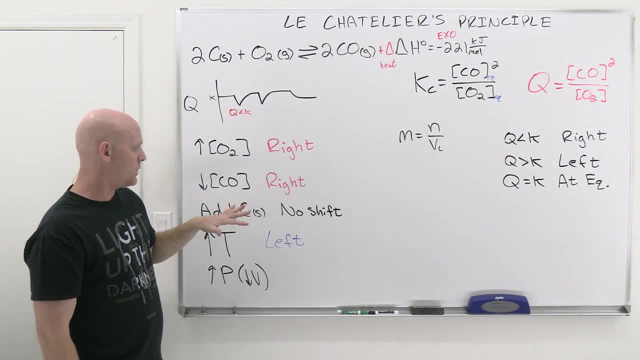 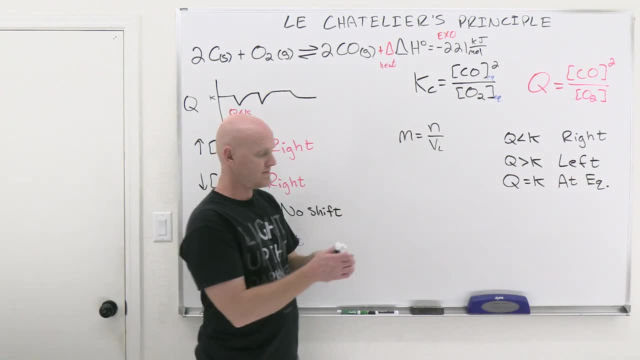 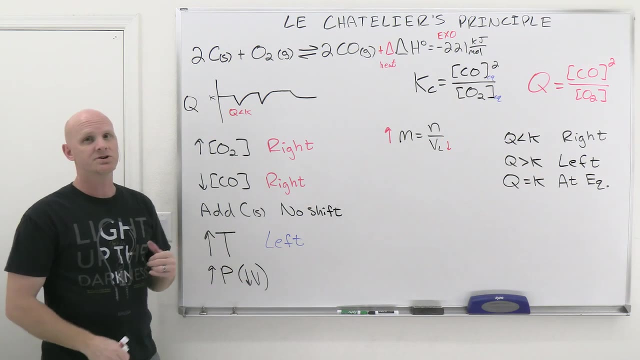 So the way this works, when you lower the volume, lowering the denominator of molarity here means you just made the molarity go up. So lowering the volume caused molarity to increase. So by lowering the volume ie increasing the pressure. 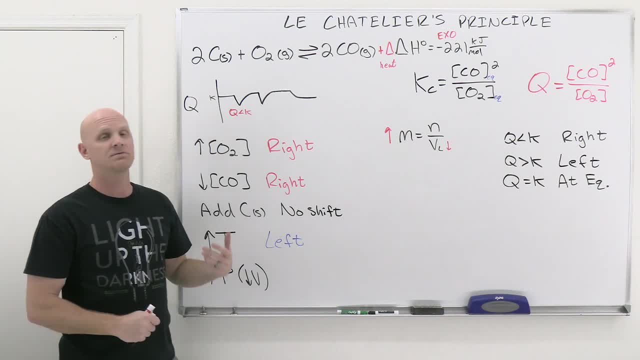 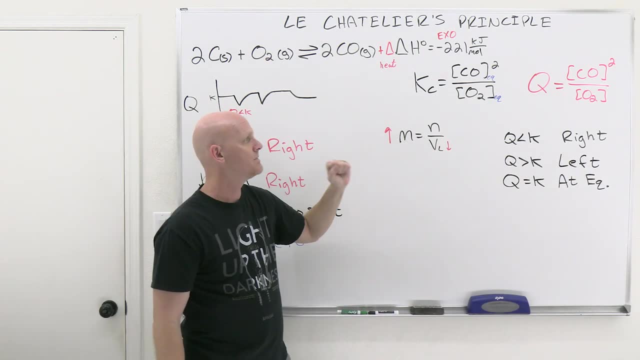 all molarities go up. And let's say you, just you know, for example, let's say you cut this volume in half. Well, by cutting it in half, you just doubled all the molarities. You doubled this molarity. 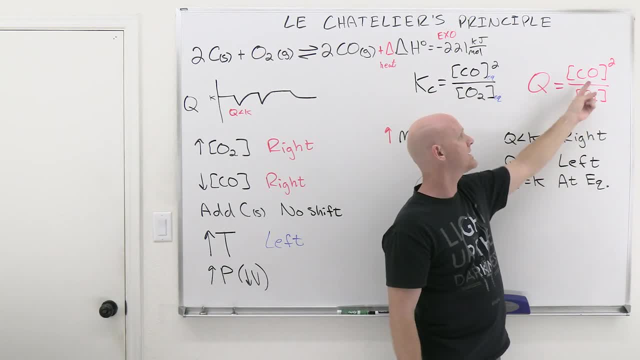 and you doubled this molarity. So it's not equal to k anymore, It's equal to q. You doubled this molarity and you doubled this molarity. Well, if you double this value and double this value, shouldn't it still be the same number? 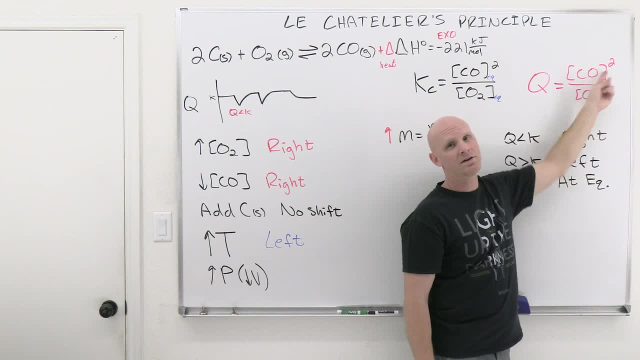 No, not necessarily, Because the top one is squared, The bottom one is not, And so, as a result, doubling the numerator and doubling the denominator, the numerator gets doubled squared, And so, overall, your q just went up in that case. 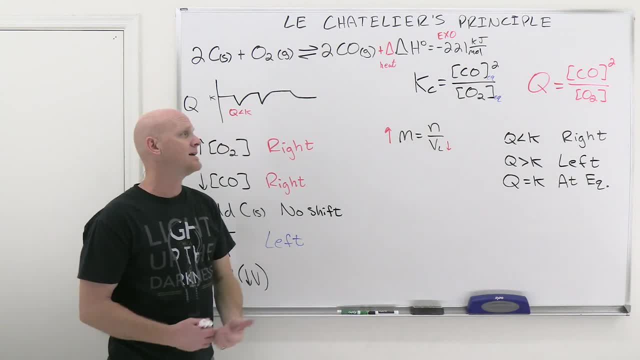 And so, as a result, if your q goes up, you're not at equilibrium anymore, And if you're not at equilibrium anymore, you're going to have to shift, And so, in this case, we'll see that. you know, if our numerator went up faster. 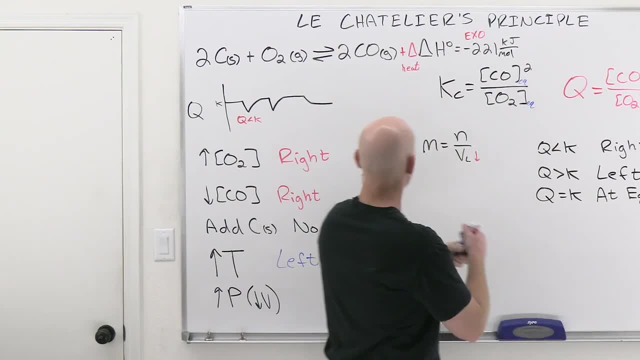 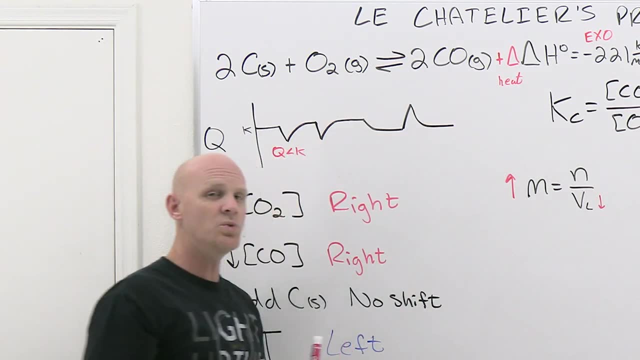 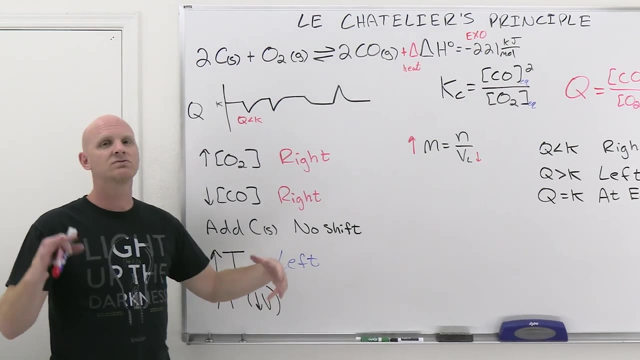 than our denominator. the numerator is too big. So, and again, q just went up and it needs to get back lower to reach this new equilibrium at this new temperature kind of a thing. Cool. Other way to kind of look at this is that if you have less volume, 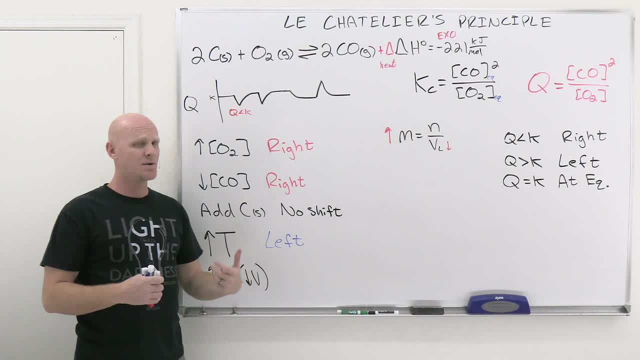 well then shift to the side that has less moles of gas, because gases take up most of the volume in your reaction. Solids and liquids take up very little volume compared to gases. Gases, that kind of normal, you know. atmospheric conditions. 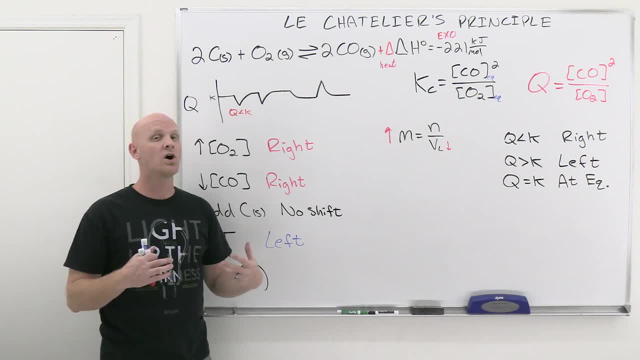 take up roughly, you know, 1,000 to 10,000 times more volume than solids or liquids. Molecules are really spread out in a gas, And so, as a result, here we've got one mole of gas on the reactant side. 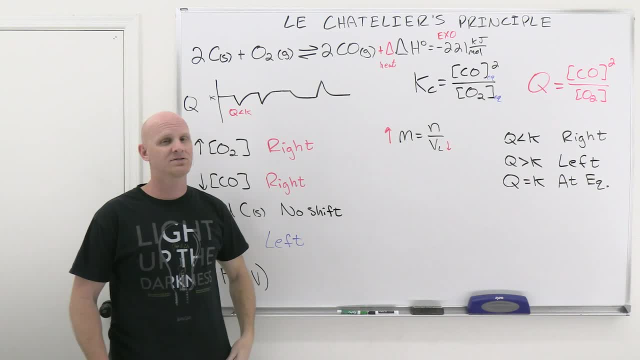 Ignore the solid. We got two moles of gas on the product side, And so if you do anything that causes a shift to the right, you're going to end up with more gas and you're going to need more room for more gas. 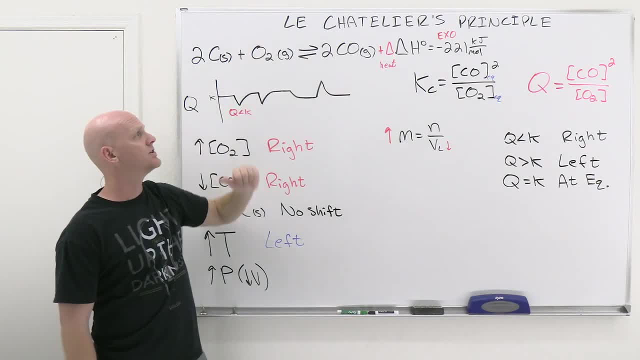 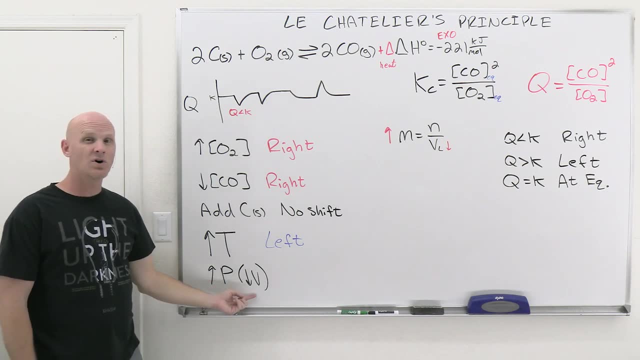 Whereas if you're going to shift to the left, you're going to end up with fewer moles of gas, which is good if you have less room available, And so, in our case, with less volume available, less room available, we definitely want to shift. 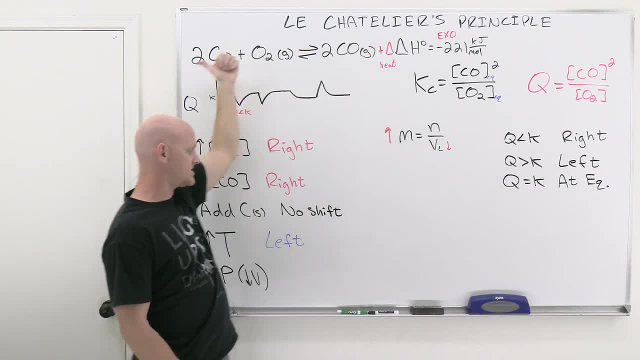 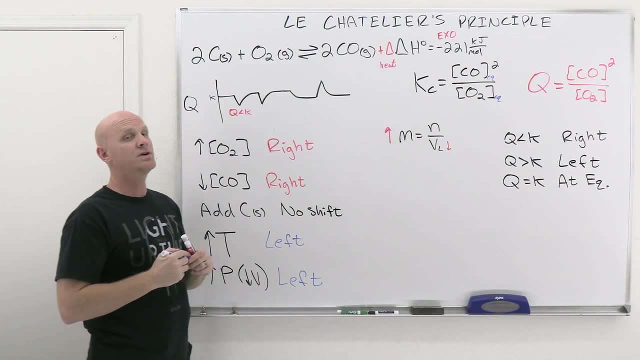 toward the side, with less moles of gas, which is going to be that shift left in this case. So that's your other way to look at it And again, if you could reason it out and be like, well, by lowering the volume. 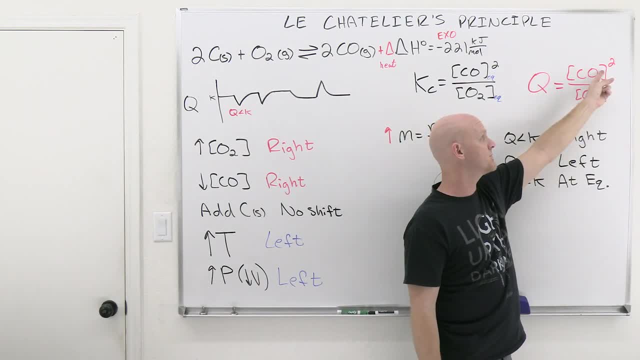 we increase all molarities, And if we increase all molarities, the one with the most molarities in the case numerator versus denominator is going to increase the fastest, And so in our case the denominator definitely goes up. 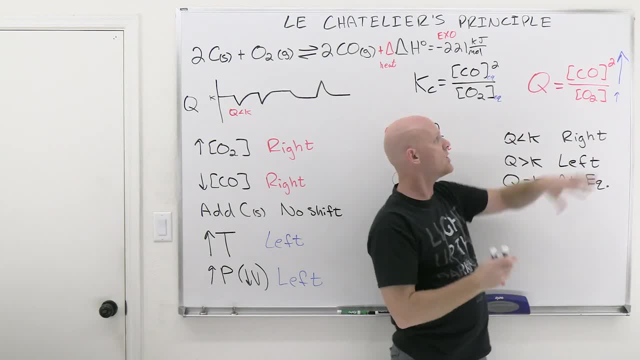 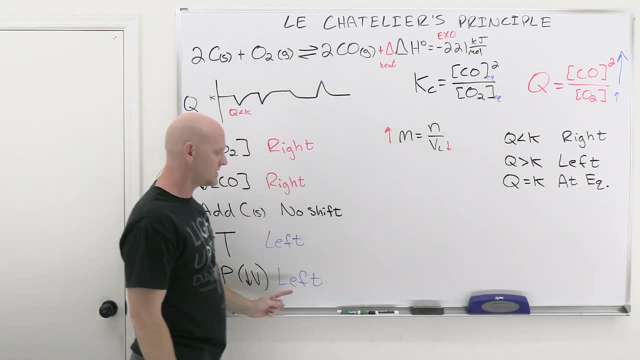 but the numerator went up more, so that overall a ratio got higher. And so if the ratio got higher then it's going to have to decrease to get back to equilibrium And to decrease that ratio we got to shift left, Cool, So that one's tricky. 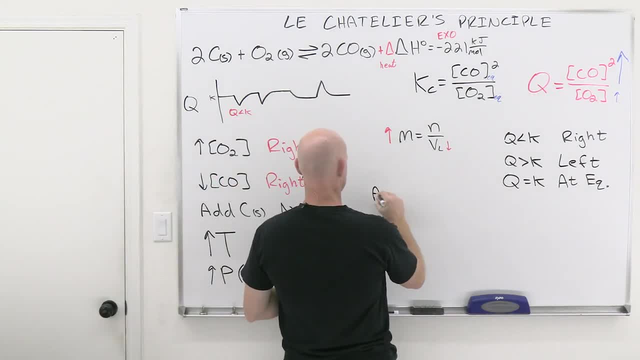 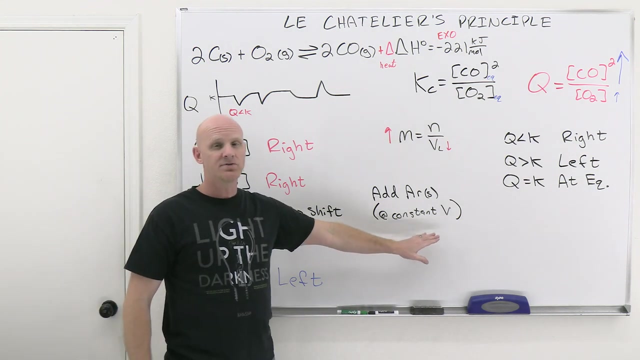 Now the last tricky one here Is: we're going to add argon into our container. We're going to do it at constant volume. So we're going to say that our container is a rigid container. It's not like a balloon where it can expand. 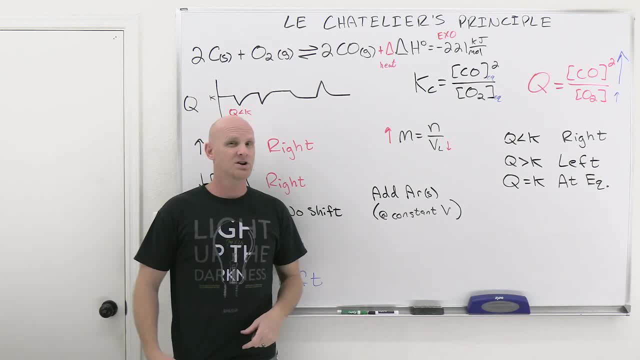 and get bigger as you add more gas into it. It's a rigid container. We're just adding more argon, And this is going to be tricky, because if I put a bunch of argon gas in a rigid container, what's going to happen? 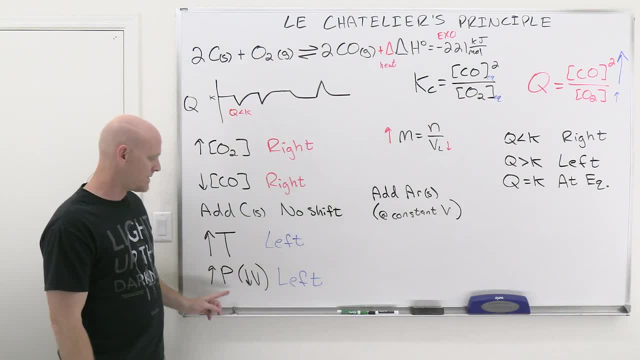 to the overall pressure. It's going to go up And you might be tempted to look back here and be like, oh, what could happen over here, Chad, when our pressure went up? But it's because we reduced the volume. But here, 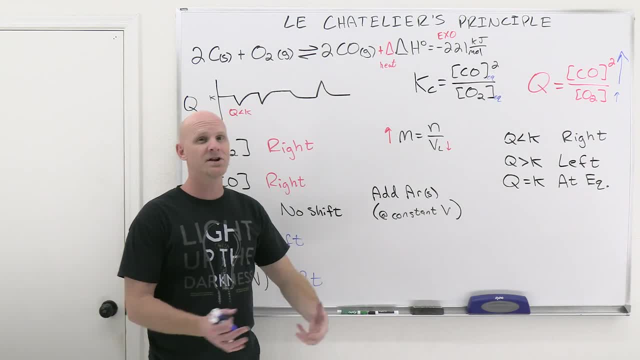 our pressure is going up, not because we've reduced the volume, but I've just added a bunch of another gas, And not just any gas. I added a noble gas, And the key here is that a noble gas is chemically inert. It's not going to react. 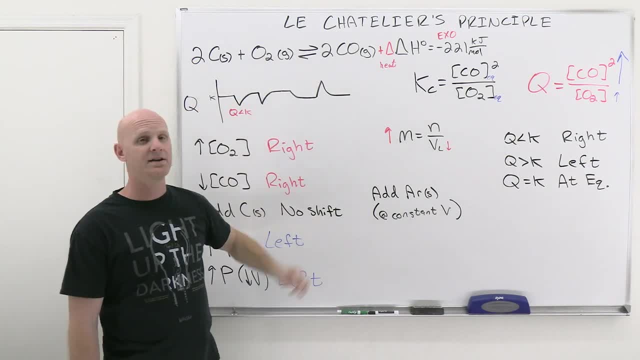 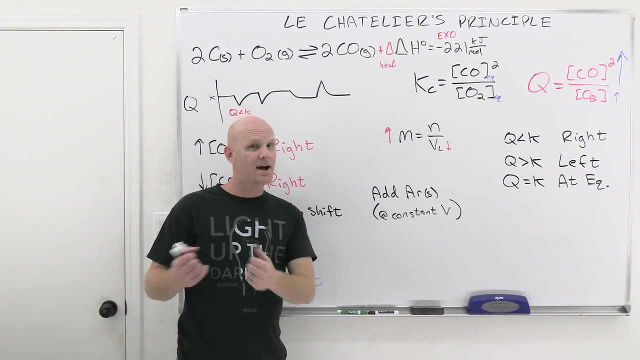 with any of the stuff in our reaction, because this doesn't do really any chemical reactions here, And so adding an inert gas which is typically going to be one of your noble gases, maybe nitrogen gas. N2 gas is pretty inert as well. 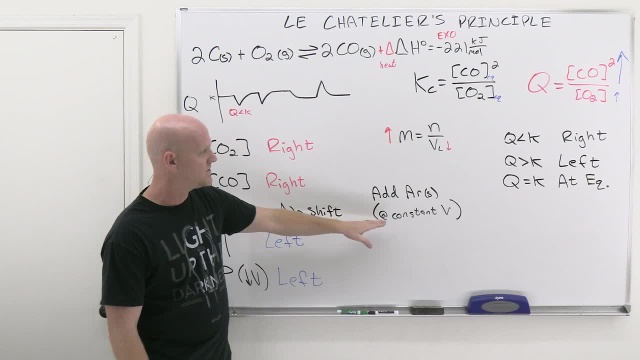 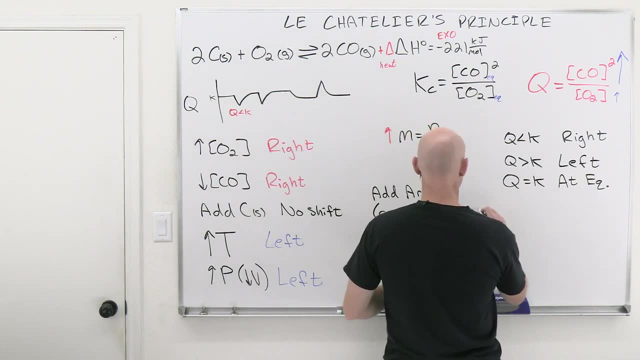 but most of the time you're probably going to see a noble gas. If you do that at constant volume, it will change the overall pressure in your container. However, you're not going to get a shift. There's going to be no shift. 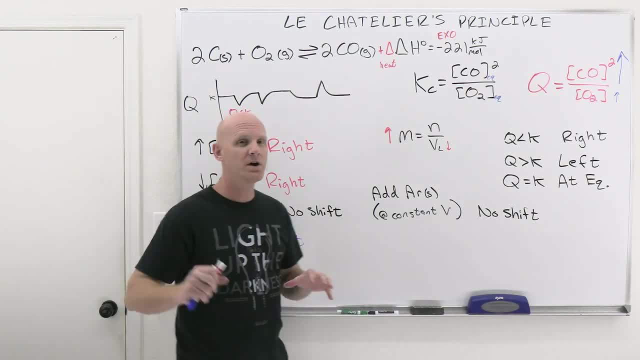 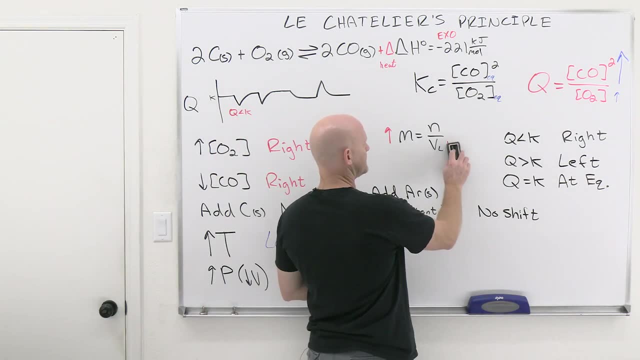 and that might be a little bit tricky. but if you take a look here, by putting a bunch of extra argon in, it did change the pressure. However, by adding a bunch of argon again, did the volume of your rigid container. 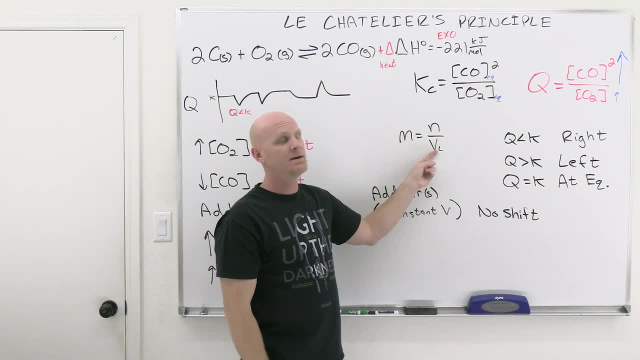 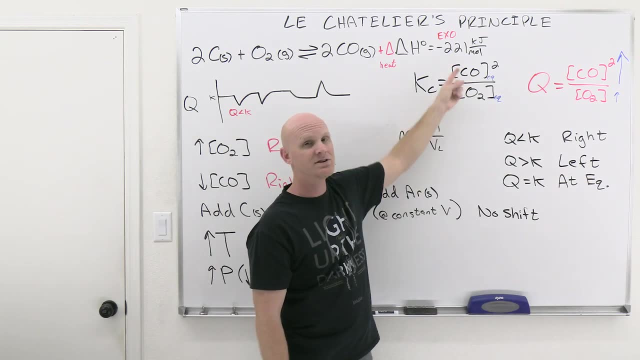 change at all? No, And if the volume doesn't change, well the moles of your stuff didn't change either. so molarity changes are not changing. And if your molarity haven't changed, then this ratio hasn't changed either. 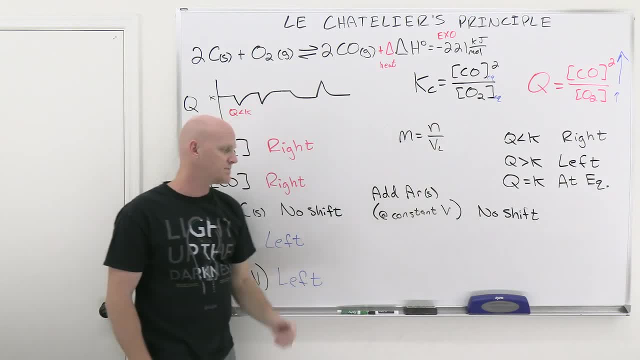 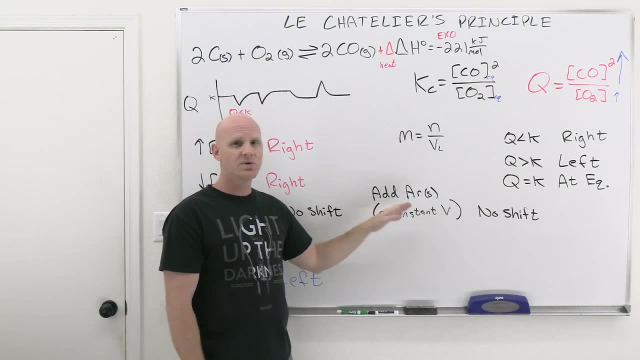 and you're still at equilibrium, And so we've got to be careful. If you increase the pressure by lowering the volume, that changes molarity and you're probably going to see a shift. But if you increase the pressure because you added an inert gas, 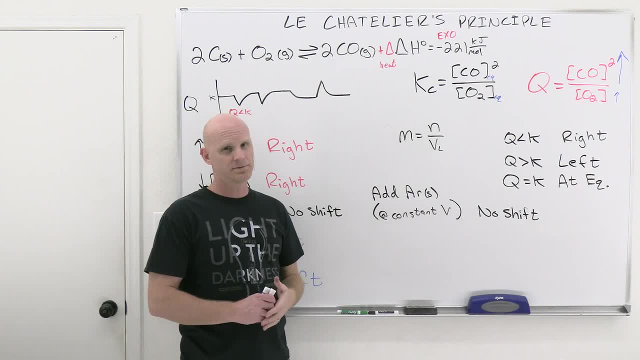 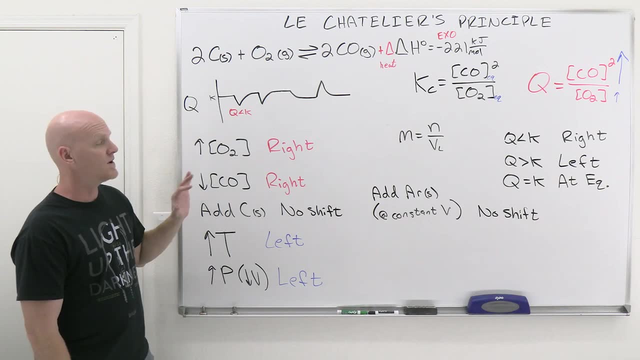 at constant volume, that's not going to result in a shift at all. Now one last thing here, and I meant to mention this back when we went through this: If you increase the pressure by lowering the volume, so it's going to shift. 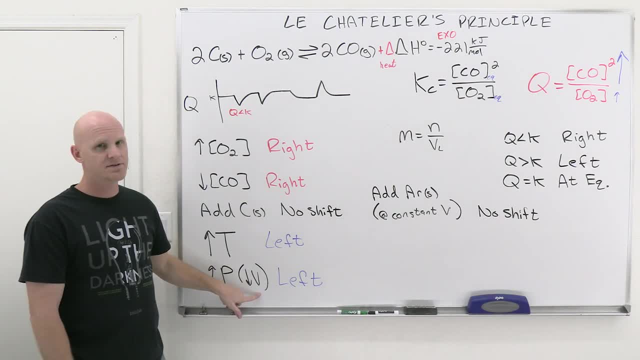 toward the side with fewer moles of gas. So less volume shifts to the side with less moles of gas, So higher volume would shift to the side with more moles of gas. It works both ways. So I like correlating your shift.